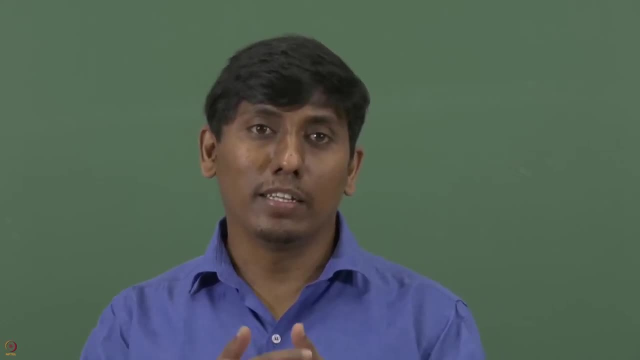 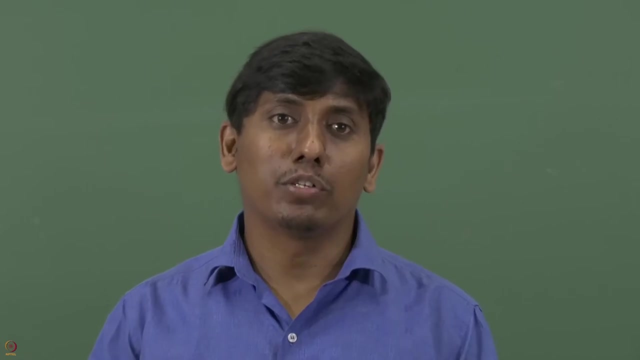 I told that we would be talking more about kinematics in the third lecture, So that is what we are going to focus here. So in this particular third lecture, we would be more focus on what is land-based mobile robot. So what would be the kinematic? 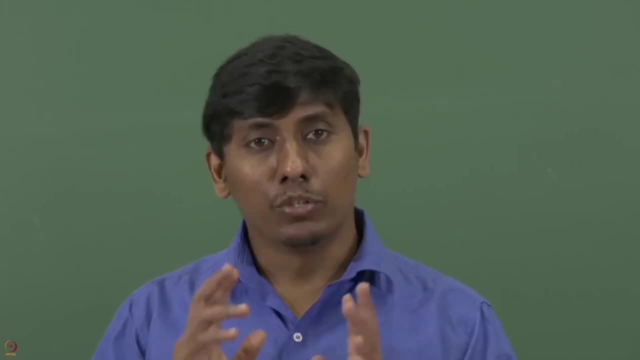 relationship, So how we can obtain that kinematic relationship. So, based on the kinematic relationship, how we can actually go forward in the further robot kinematic aspects, For example forward and inverse differential kinematics. So in that sense, as we 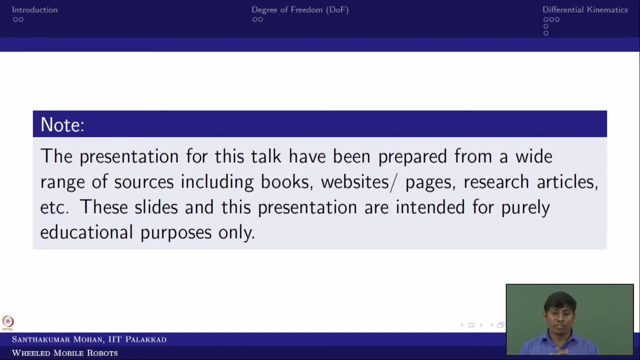 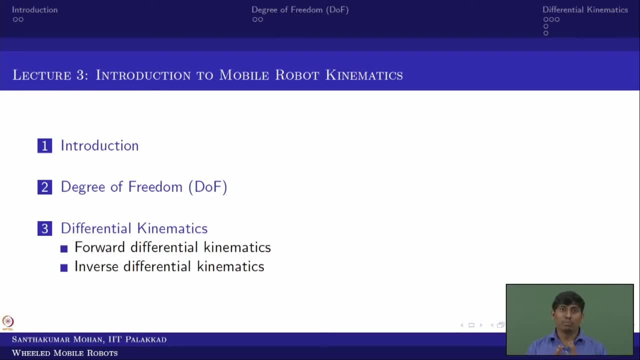 did in the last two lectures the similar way. So this is the note. So let us move to the particular topic called lecture 3 in this way. So this particular topic or lecture would be focusing, as I already mentioned, it would be focusing mainly on the mobile robot kinematics. 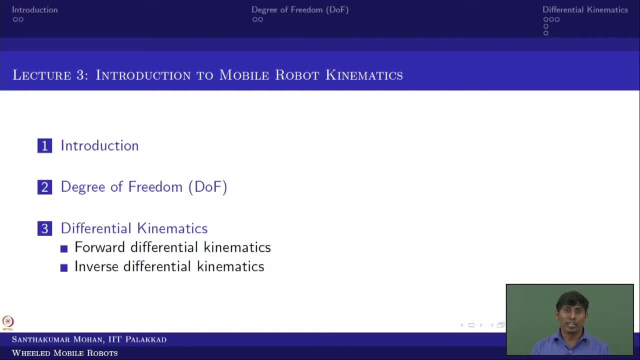 As I already told, mobile robot means in general it is a land-based. So land-based means it is actually like having you call planar movement, So we will not be seeing the off planar movement. So that is what the overall idea. So let us start with the. 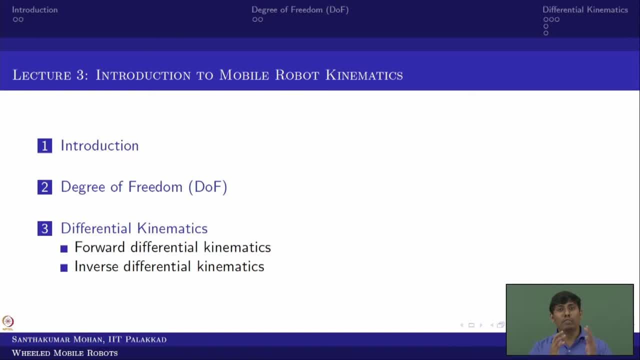 basic introduction about mobile robot kinematics, and then we move forward to what is degree of freedom and what is differential kinematics. So this is what the overall flow which we planned for this lecture 3.. So let us start with the kinematics. So kinematics, you already know it. 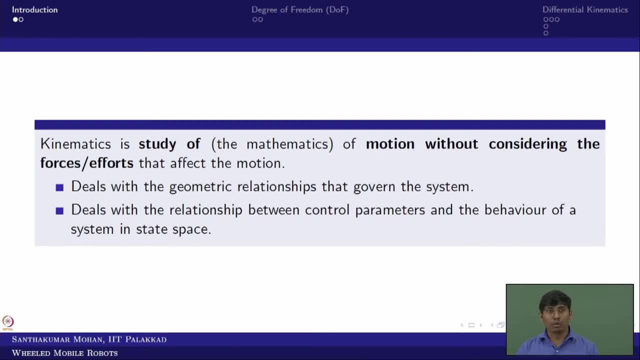 is one of the branch of you call physics, So where you talk about statics and dynamics. So inside dynamics, you know one of the- you can say- subsection called kinematics. But what this all means is that the relationship between the forces of the motion and the moments. 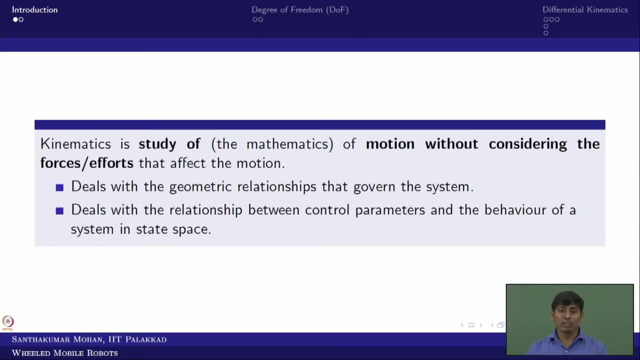 So what kinematics is? you are in a relationship with the motionn on our head, With the motion, because if you helps this force, we can see only this motion, And if the force is not ‑‑ if the force goes further, then we have very littleivity. Can you show me the force or the motion on the head? 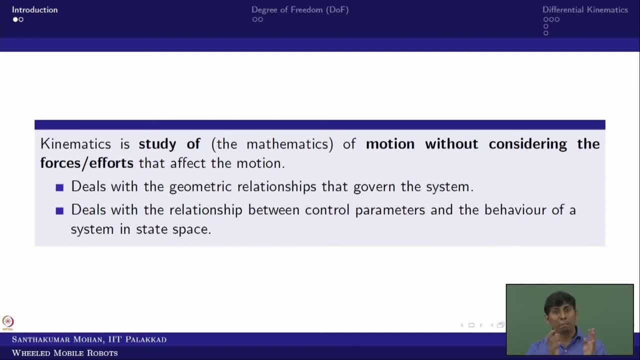 So doing that, we are in a relationship with this motion, with this vis Tes, Which brings attraction bonding by attraction bonding, since the force onde and the motionI am such, the two spaces or we are trying to map between the input and output. 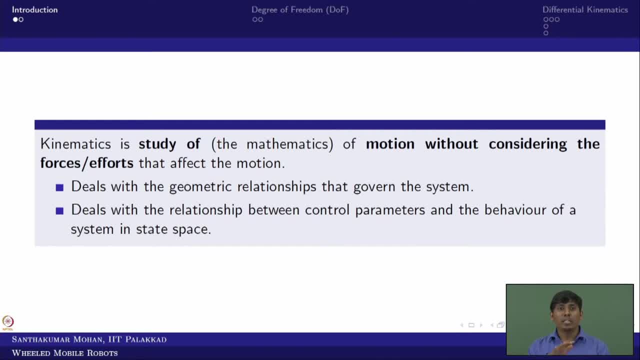 Although here the input is not force, or you can say moment, but the input in the sense, the control parameter and the system parameter, what you call motion parameter. we are trying to make a mapping. So this mapping, what we call kinematics in robotics, 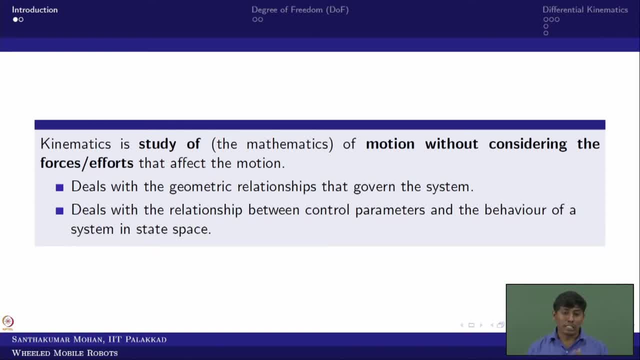 So that is what we are trying to cover, As I already mentioned, you can see that kinematics what it deals with, the geometrical relationship that govern the system. So the other one is it deals with the relationship between control parameters and the behavior. 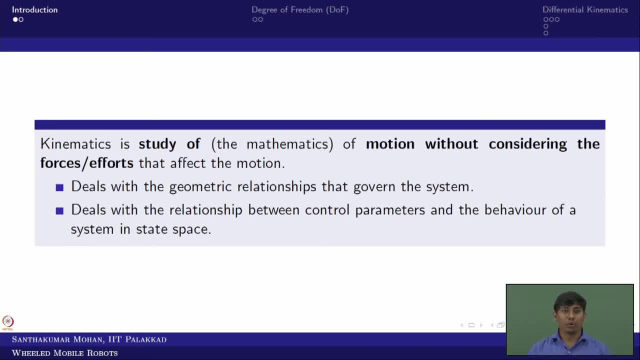 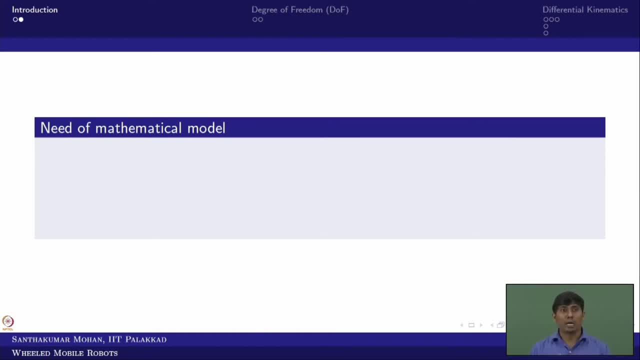 of the system in state phase. This is what actually like one important thing. So let us actually like move forward in that case. So why it is required? So the kinematic model or mathematical model, why it is required, There are three purposes which we are putting forward. 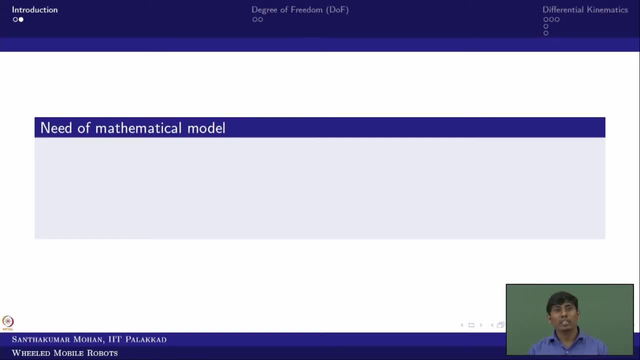 So one is actually like to understand the system. So definitely. so what kinematics means? it is study of motion. So in the sense we are trying to understand the system, motion. So that is one thing. Second thing is what happens? so if you are study about the motion, so what one can see? 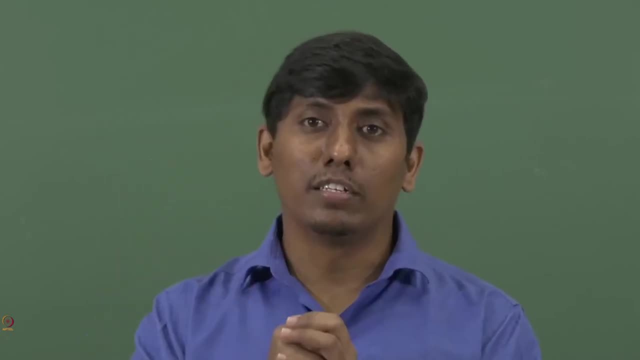 you can actually like see how to design that particular system. For example, if I actually like make a two wheel mobile robot, So how that two wheel supposed to be located, Whether this is what the length, or you can say the distance between these two wheel, I 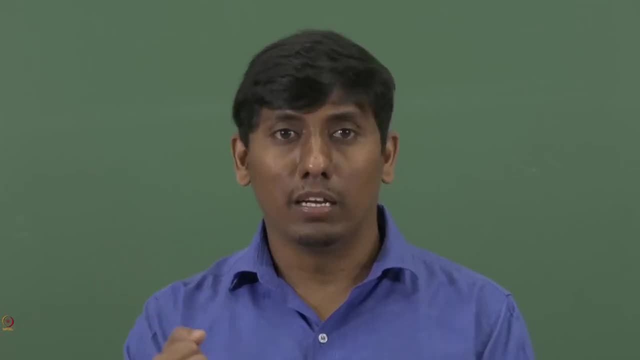 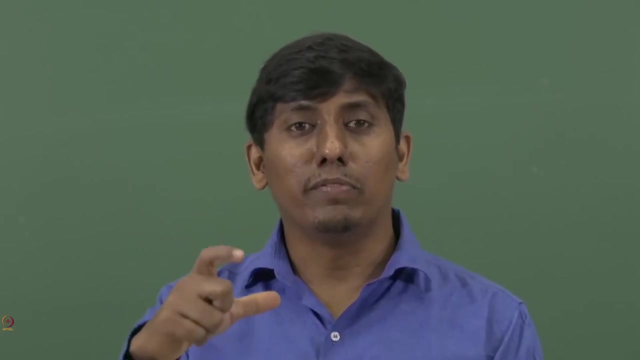 need to put it like this. For example, now you take it as a cycle bicycle, So the front wheel and the back wheel, if I have probably the length, or you can say the distance between these two wheel, so that parameter change, the overall system study. 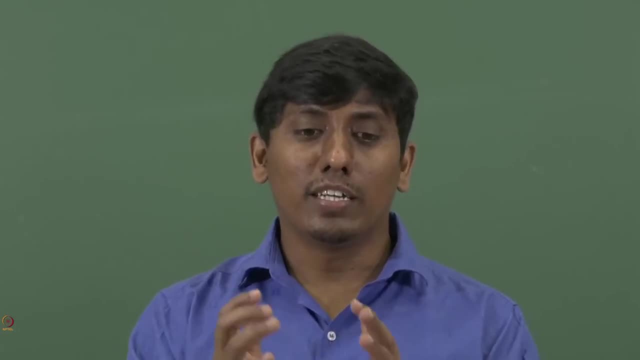 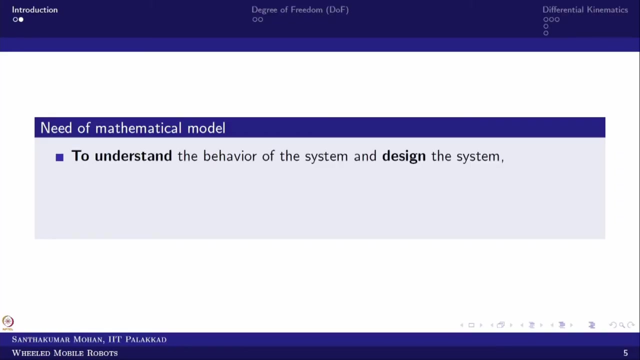 of motion right. So in the sense you can actually try to do, In that sense you can see the need of mathematical model come the broad way. so, which is nothing but the to understand and design the system, right To understand the behavior of the system and design the mechanical system. that is what 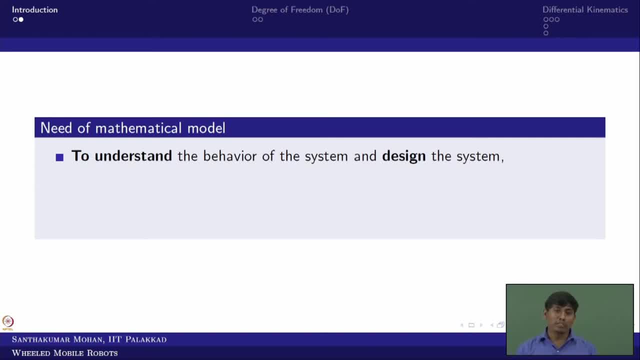 I mean to say here the locomotion system. The second point is very straight forward, since I already told, the kinematic model is deals about the you can say relation between the control parameter and this, the system parameter, In the sense, what you can see this mathematical model can be used for. you can say design, the, 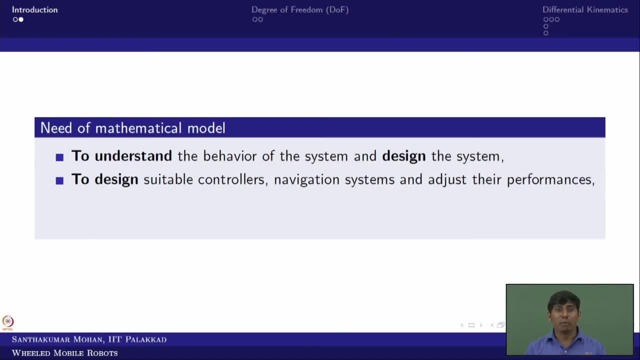 proper motion controller. Further what you can see, since it is a mobile robot, even we can extend for navigational system design and there you can say performance tuning. So these are actually like two broad category. Any mathematical model for you can say mathematical model of a robot. definitely these two are. 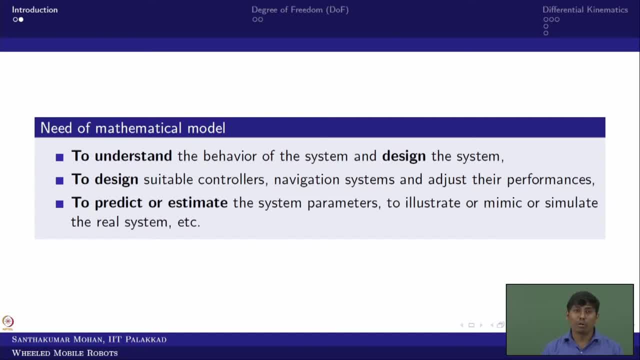 the primos. The third thing, which is actually like very one of the important thing, very you can say specific. we can actually try to. you can say predict or estimate the system parameter. For example, you take a car- the car I am assuming- in kinematic, or even you take a general. 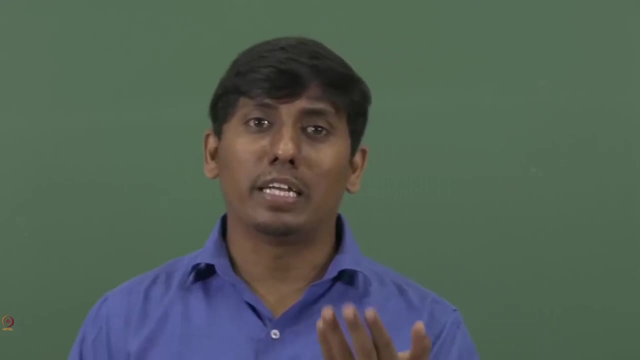 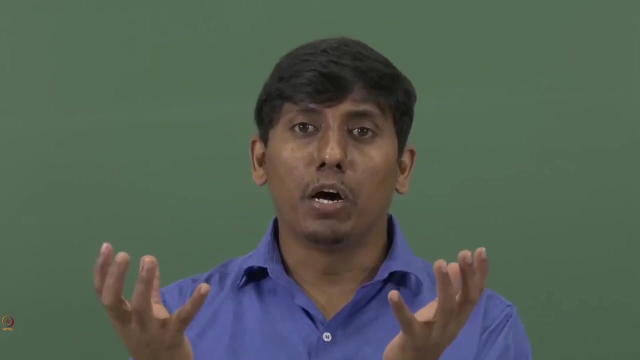 thing, certain parameter you cannot actually like measure or estimate. you can say accurately. So then what we can do, we can actually like use a mathematical model which is, you, predominantly based on the first principle, Right? So you can actually like adjust the parameter based on the real. you can say output and as 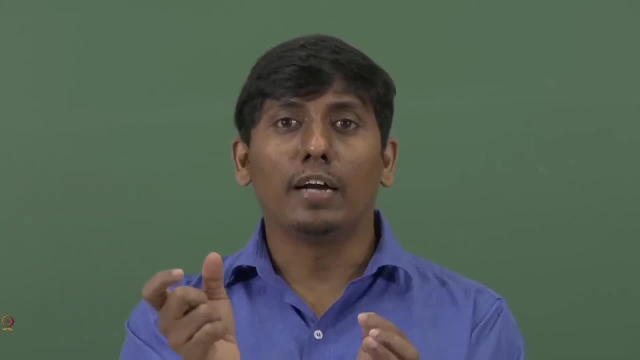 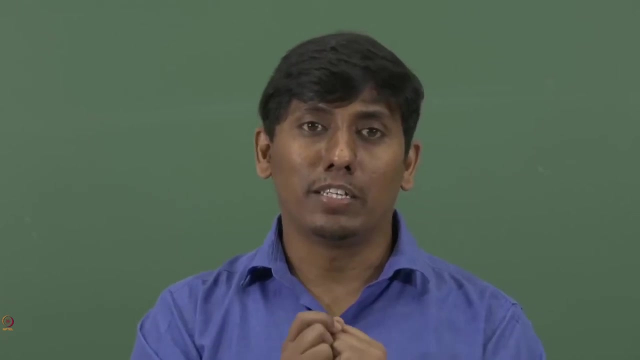 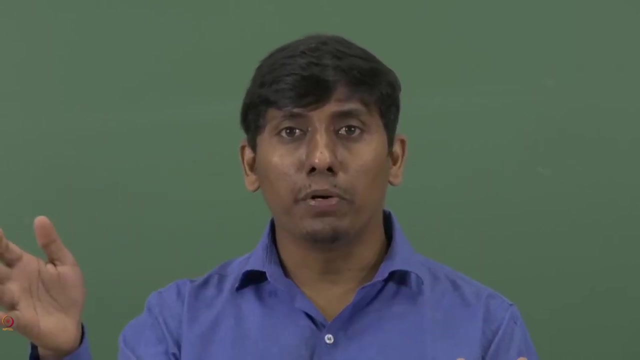 well as your model performance. You can see, you can actually tune and you can actually like identify In the sense what people call it is can be used for system identification or parameter estimation, For example. you take in the other way round, So you take a open system and give input and take output. 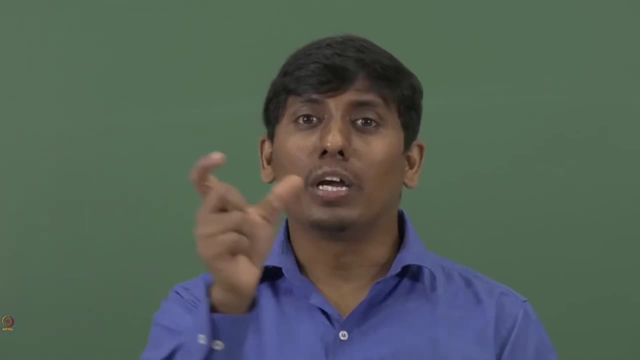 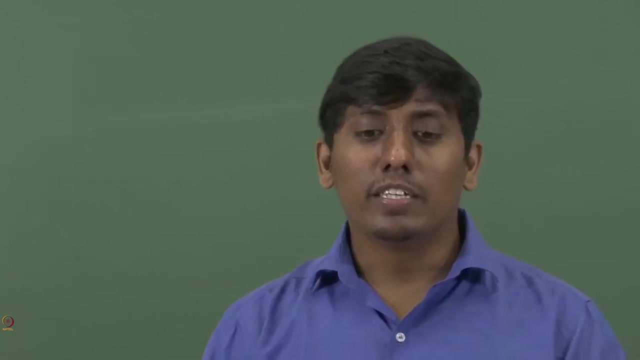 So what one can see from the input and output relationship. you can understand the system Right. So what would be the system? So that is what we are actually saying: that to predict or estimate. in the sense, the mathematical model definitely can be used for these three purpose: to design, to understand. this is the 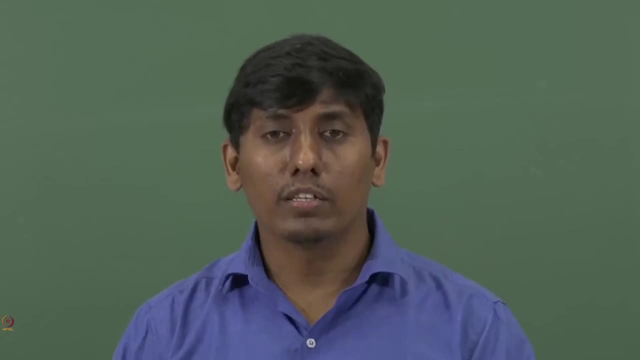 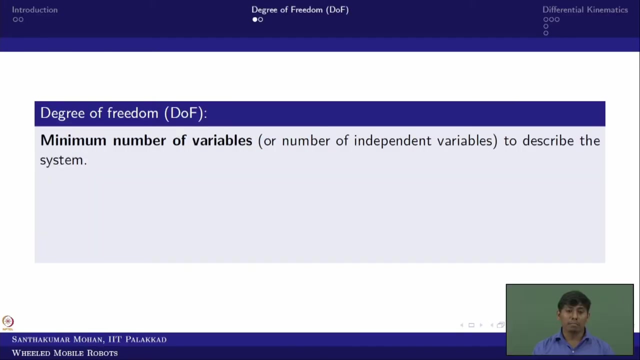 combined fact and to design controller. this is another fact. and the third fact which we call to predict and estimate. So now we move little forward. So what that mean? So we will talk. the mobile robot kinematics. So for that, one of the important thing. 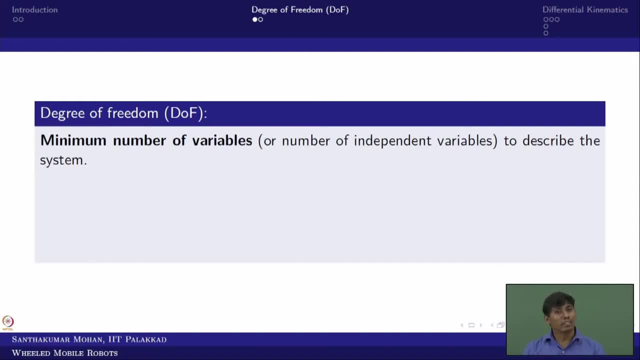 So what that? So, for example, now you are talking about the description. So what that means. So what is the description? That is what? nothing but Right. So what the description? So you are going to describe the motion. 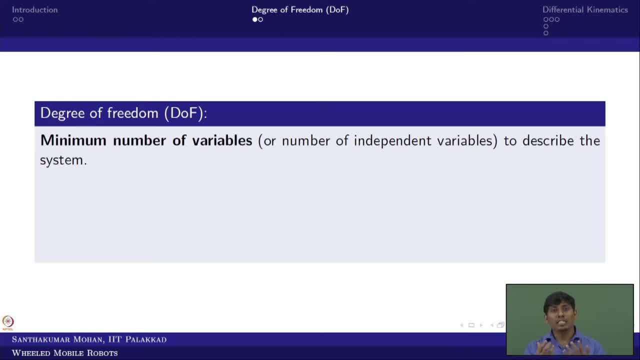 So now, in order to describe the motion, you have to see certain parameters Right. For example, you want to describe about me, Imagine, So you know, like one of the faculty in your institute he come from probably IIT, Indore. 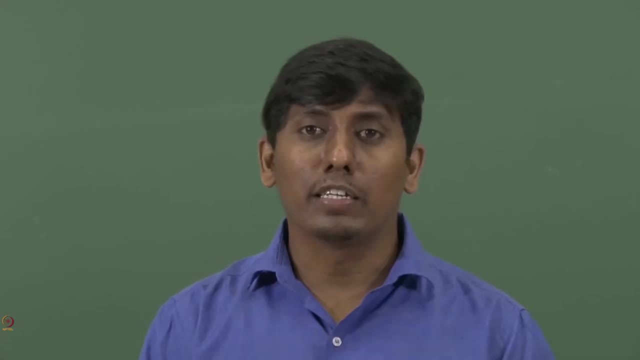 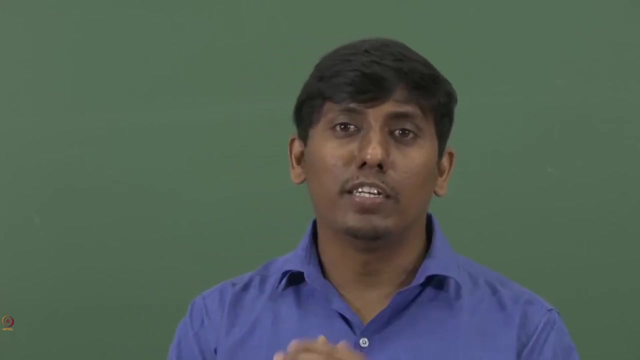 Imagine: So I was working in IIT Indore, for example, 7 years I was there, So now you forget my name somehow, But you are actually, like, know some of the credentials of me. So the person who is coming from IIT Indore definitely put that credential. you can understand. 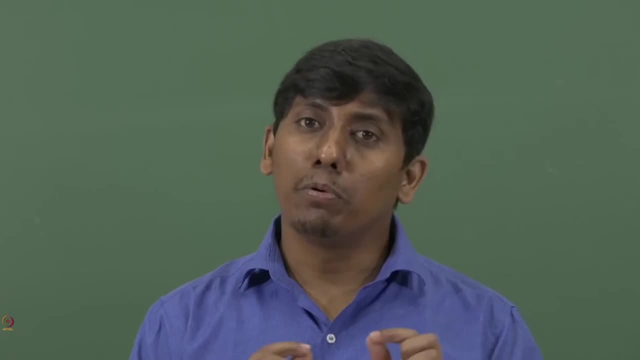 Now for putting that credentials, you have to put the minimum number of. you can say credentials. For example, you can say that the guy actually, like, worked in mechanical. you want to describe me? Okay, this is one credential. Second thing is he graduated from IIT Madras. 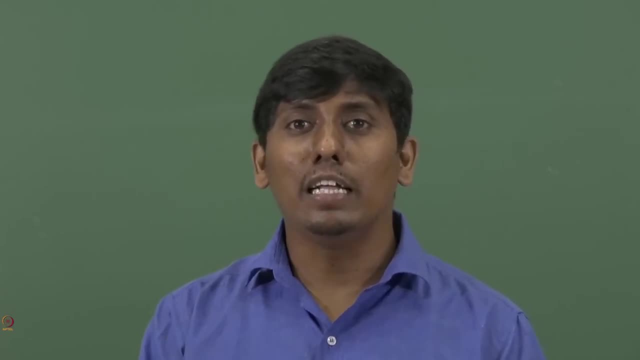 Then you can see that even in IIT Indore currently there are four faculty working in mechanical engineering who graduated from IIT Madras. These are not sufficient, Right? Then you put another keyword: probably he is working in robotics. Then also you can see that in IIT Indore there are two professors are working in robotics. 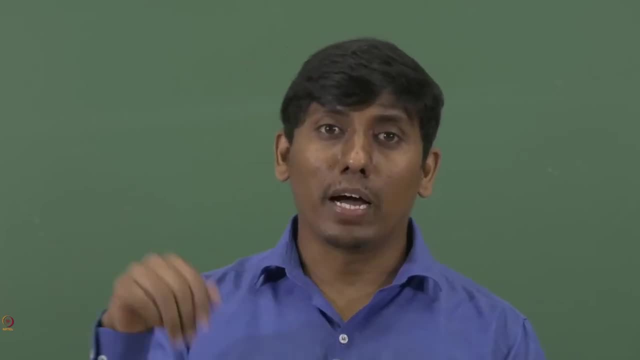 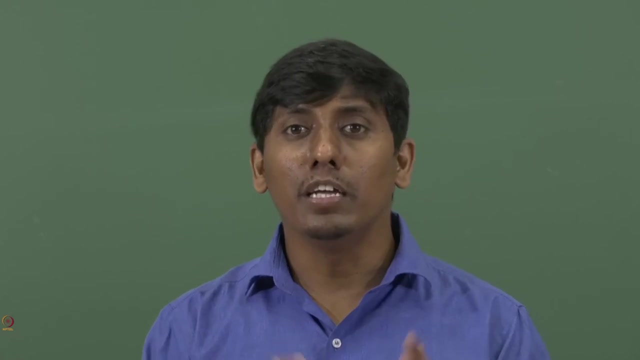 Then that too, like from IIT Madras itself, Then you can actually put one more credential. You can say that this particular person who was actually like in Germany for more than a year, Then you can see that the person who is actually like listening in the other side, he can understand. 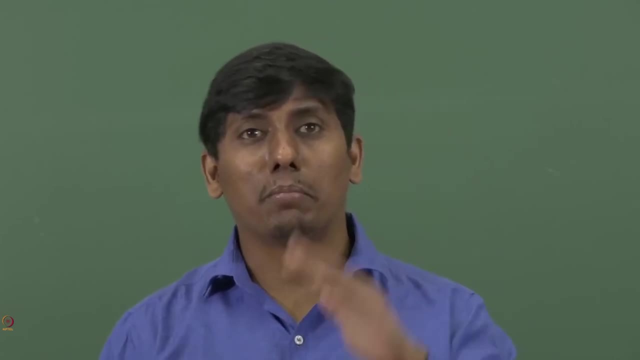 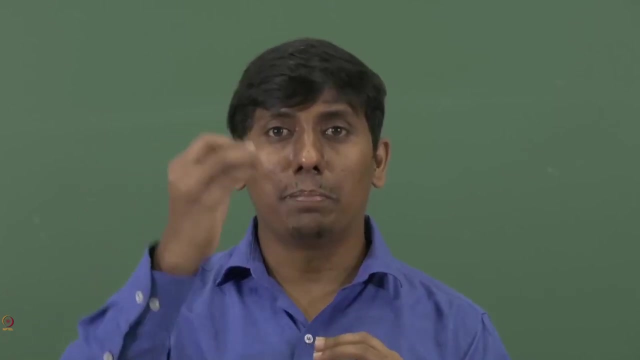 Oh, this guy is talking about Shantak Mara. Okay, now I got it. So now what you put? You put a- you can say- list of description in such a way that the opposite person can understand and identify the- you can say the current person. 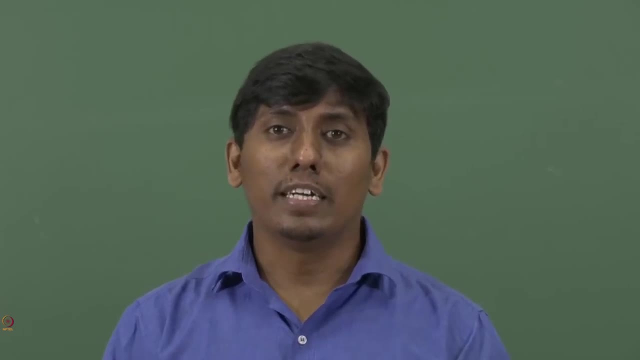 So now, the same way, when you talk about, you can say description. So when you talk about the study of motion, the motion description. So how many variable required to describe in a unique way? So this is what we are calling as a minimum number of variable to describe the system. 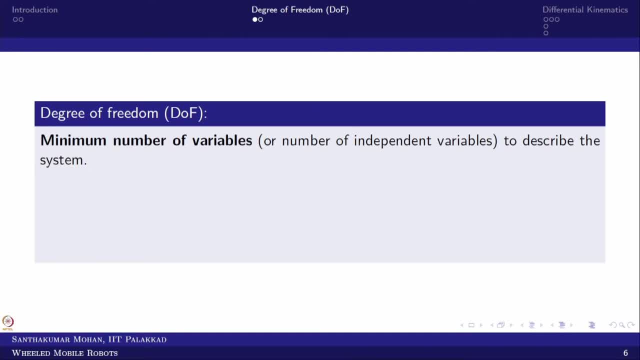 This minimum number of variable, What we are going to call as degree of freedom. Why it is called degree of freedom? Because we are talking about the system which is in moving. So what are the possible motions, or what are the possible movement happened on the? 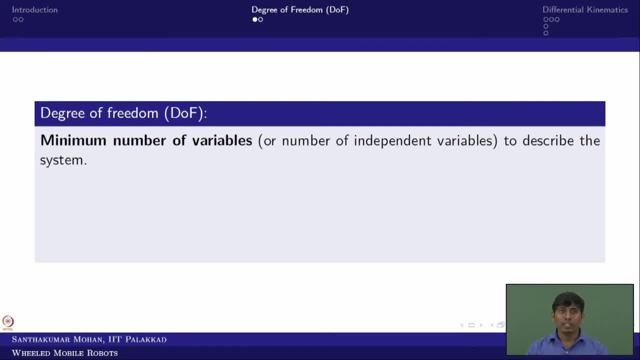 system. That is what we are trying to give a idea. So, in the sense, what? in the other way around, you can say number of independent variable to describe the system in unique manner. This is what degree of freedom? So now you got a very general definition right. 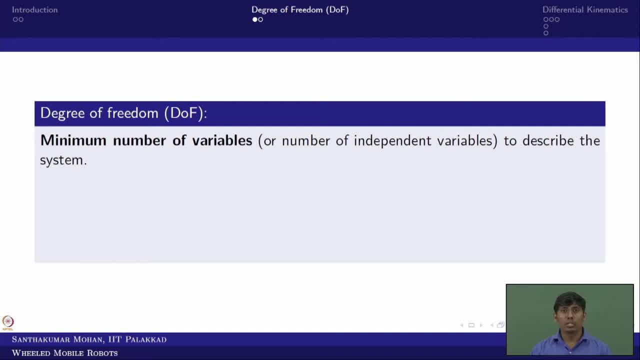 So now we can actually like see, If you talk about a mobile robot, So what are the possible motion? So mobile robot mean it is a land base, So you can see that the robot can move in longitudinal way, lateral way, and it can rotate. 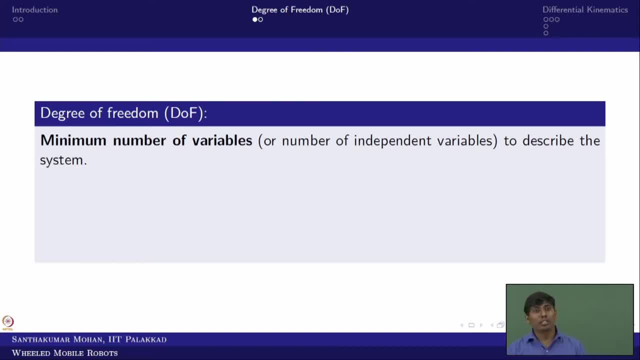 about its own vertical axis. In the sense, what are the possible motions? So there are three motions. So now, in order to describe these three motions, what are the number of parameter required? at least three parameter, right. So that is what we are going to call as a degree of freedom. 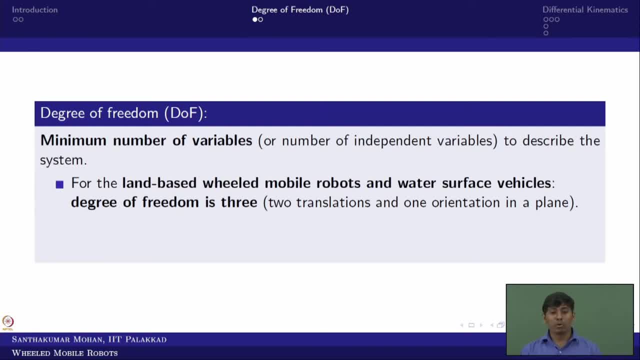 In the sense for land based, And you can say mobile robot in general, wheeled, ok, in specific wheel, And whatever you call water surface vehicle. all are actually like coming under a planar case. So we are assuming that the aft planar movement is not there. 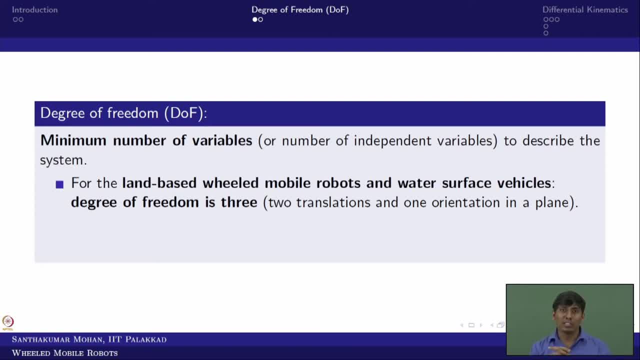 So in that sense, what are the possible motions? two translations and one, you can say, orientation in a plane. So in the sense you can see there are three motion primitives are required. In the sense the degree of freedom is three. Now you take a very general case. 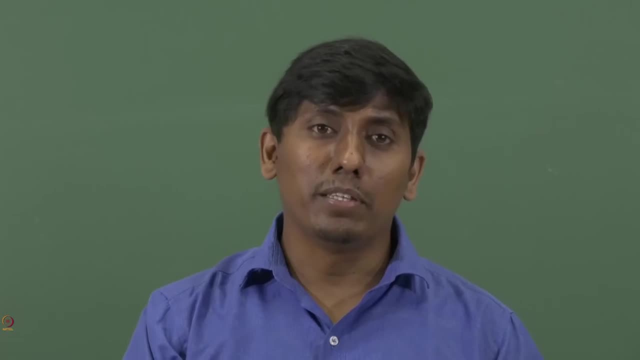 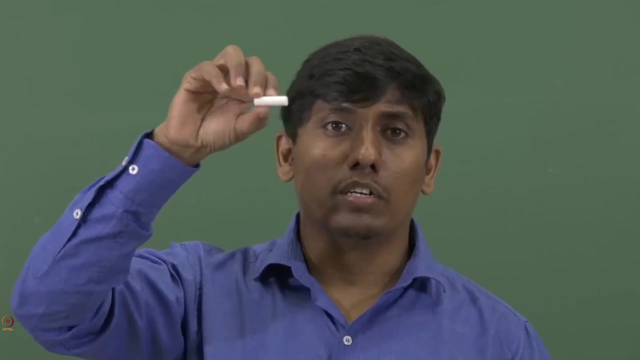 You can take a space. So now you take, for example, this chalk. This chalk actually, like, I can put it on the space. So now I want to describe this chalk motion, for example. So how many variables required? This chalk can actually, like, move in three dimensional space. 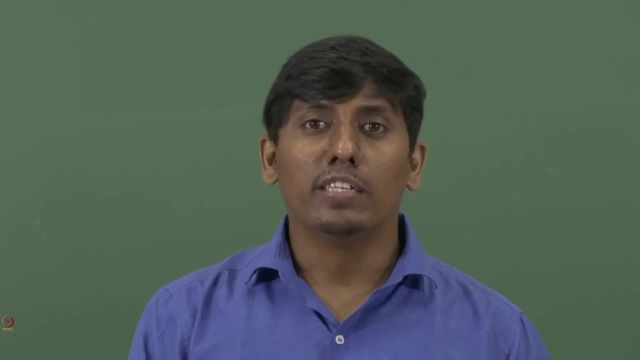 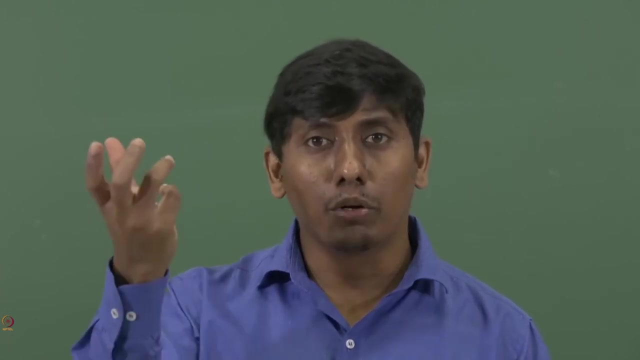 So in the sense, three translation and three orientations required. In the sense, the degree of freedom for a general case in three dimensional space it required six. So now you take a aerial robot or underwater robot or space robot, These all required actually like six parameter describe. 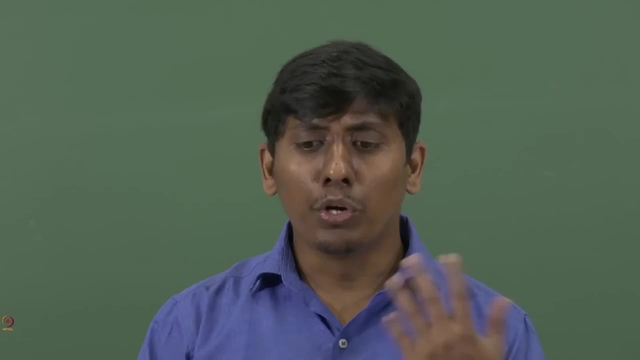 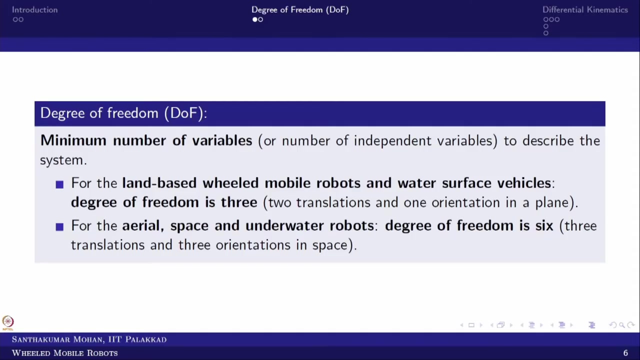 In the sense, the degree of freedom is what you call six. So three translation and three orientations are what you call actually like a degree of freedom for this particular system. So this is what we are actually like mentioning. So now you know what is degree of freedom. 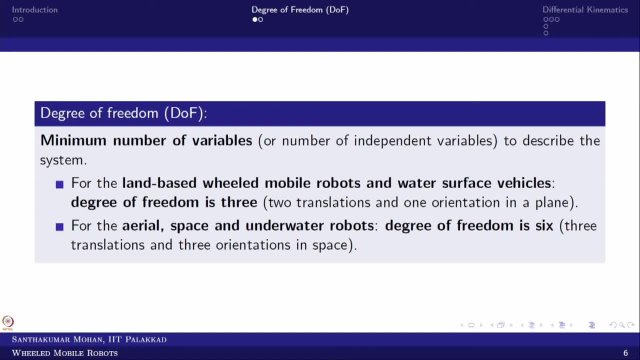 It is nothing but minimum number of variable to describe the system in unique sense. In that case we are focusing on the land base. In that sense, the degree of freedom is three. That is what we are focusing, So, in the sense, what we are doing in this particular course. 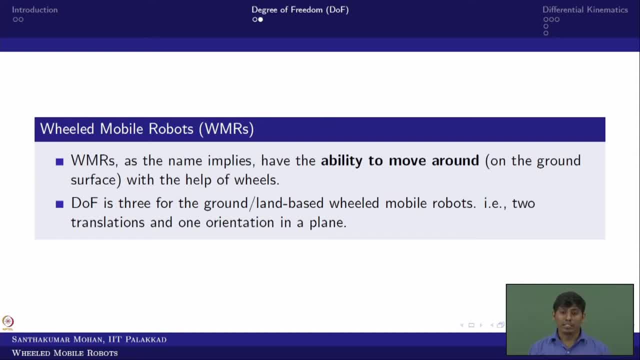 This particular course is all about wheeled mobile robot. In the sense I am putting the same keyword again, So ability, move around with the help of wheels. So in the sense, the degree of freedom in this case is three right, So now two translation and one orientation we need to describe in a plane. 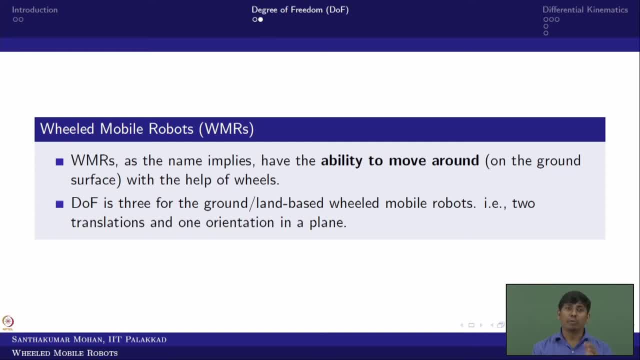 So now we are taking that into a general case. So now imagine I have a magnetic duster and there is a steel board in the beginning. So now I put that magnetic duster on the steel board. What will happen to that? 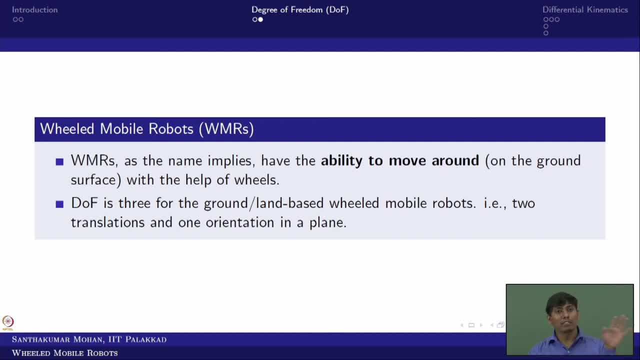 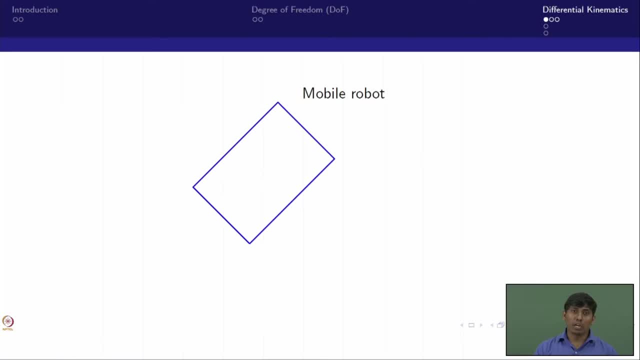 That steel board will not allow the magnetic duster come away. But if you actually like, move around. what happen? The two translation and one orientation is possible. So that is what I am trying to put it in this particular slide. You can see that this blue color box what I draw and imagine as a magnetic duster. 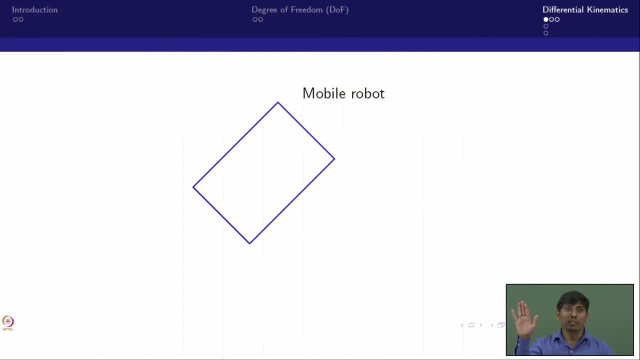 Now this magnetic duster can actually like move lateral, In the sense in this case it is longitudinal- And as well as rotate about it- right Now I call that is as a mobile robot in a land. ok, Land based system. this is a mobile robot. 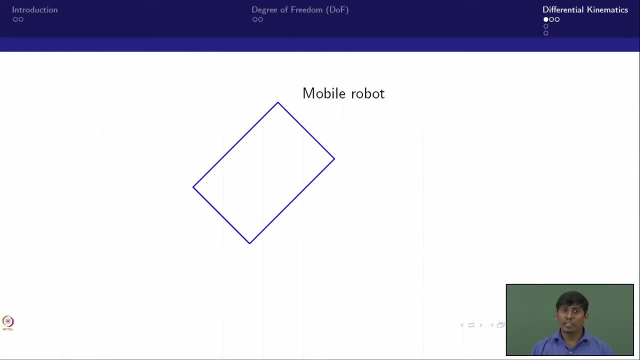 Now, in order to describe the system, what I need. So, first of all, in order to describe, some standard thing is required. For example, you are actually like describing about me, For example: brown color skin, you can say long hair, short height. 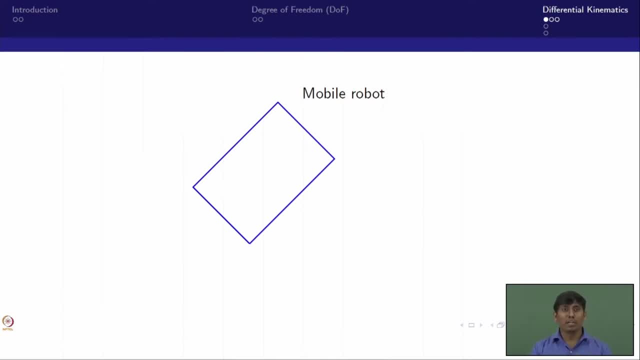 So these are description. But now the same description. if I go in a different country, For example, if I go a Mongolian country, I may not be a short height, right? If I go, probably, in a Korean country, I may not be having a long hair. 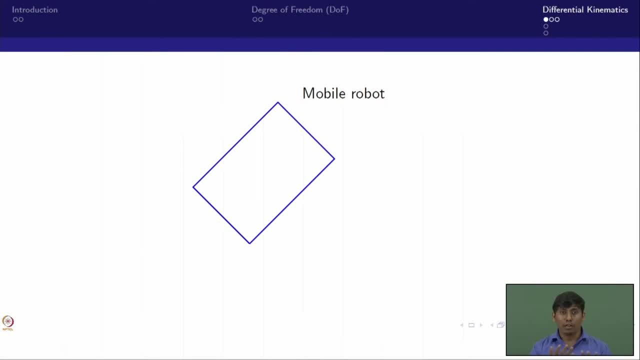 If I go probably Africa, I may not be a- you can say a brown fair right. So in the sense you can see that there is some reference you have to maintain So what that? So you need to have some reference. So in that case, here we are going to describe about the motion. 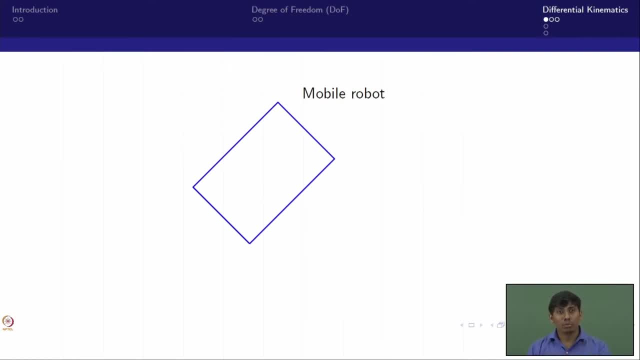 So what would be the motion? Motion can be described in two translation and one orientation. that is what here. So, in the sense, what you need to have, You need to have a frame. So, in the sense, you need to have a coordinate system. 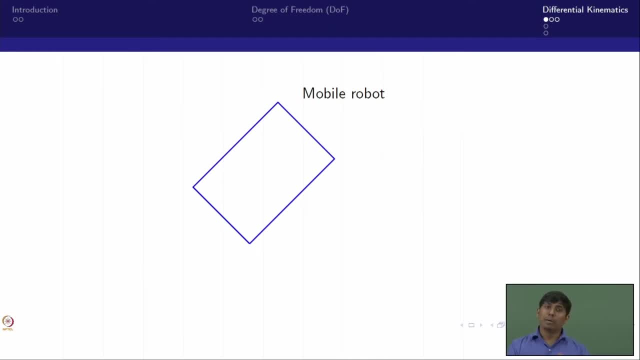 So there are several coordinate systems are possible, But we are taking one of the simplest one, which is what we call Cartesian coordinate system. There are three mutually perpendicular axis which is connected with a single point. that is what we call Cartesian coordinate system. Since it is in a plane, we can take one of the Cartesian coordinate system. here and now you take even Cartesian coordinate system. 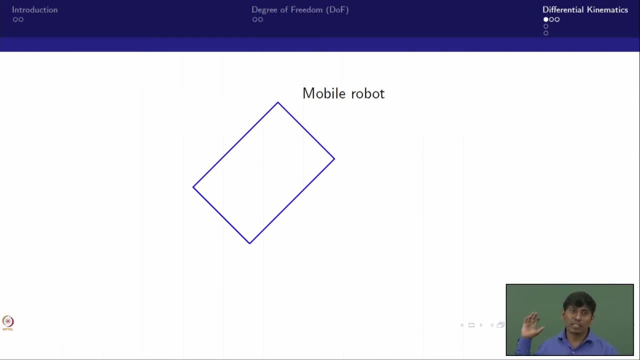 Still, I cannot define the system right, For example, if I take a duster on the board, So I need to define the position of the duster with respect to something. So for that, what I am bringing, I am bringing one of the point which I call I. 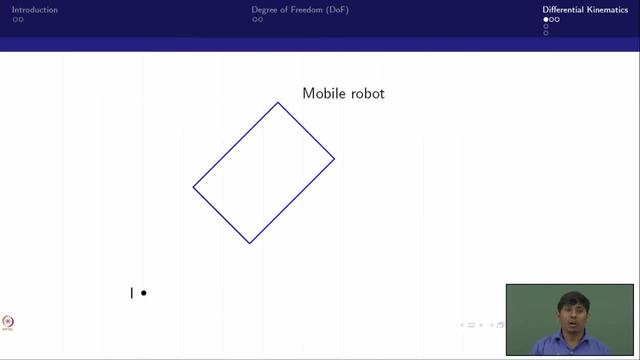 So why I call I? This is inertial, So I am going to call I means inertial in the sense it is fixed on the wall or fixed on the board, it is fixed. So now I am actually like putting the Cartesian coordinate system where z, i, in the sense z axis. 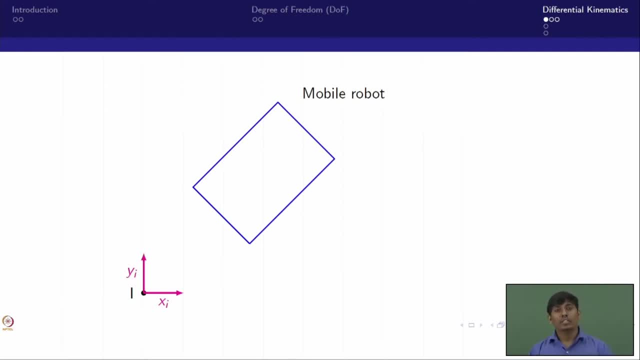 That is actually like coming out of the screen. ok, So that is what we are going to use. in that sense, we are going to use the right hand coordinate or right hand rule. So where thumb finger goes x, you can say forefinger goes y and z axis would be represented with the middle finger. 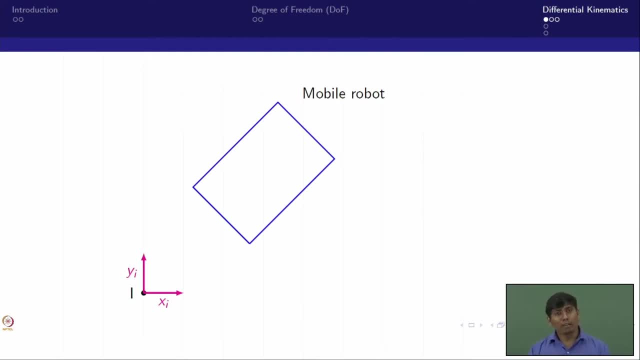 So now this is fine. So still, you may have a doubt. So how can I represent the motion of the robot here? Because this is one of the coordinate, but the mobile robot is having infinite number of points, right? So how I will define? 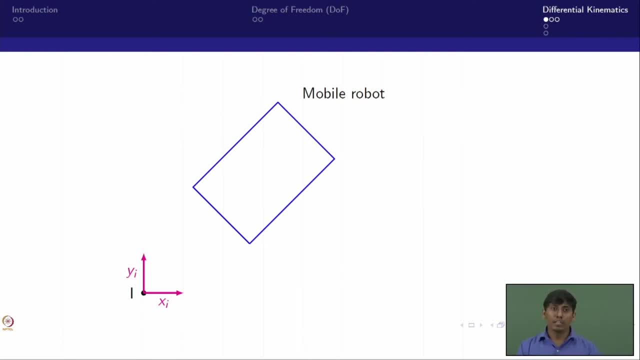 So for that, what we are bringing, one more coordinate, which is we are going to call body fixed coordinate. So this is- I am putting one of the convenient point here, which is nothing but b, That b is having another coordinate system called. you can say x, b, y, b and z, b. 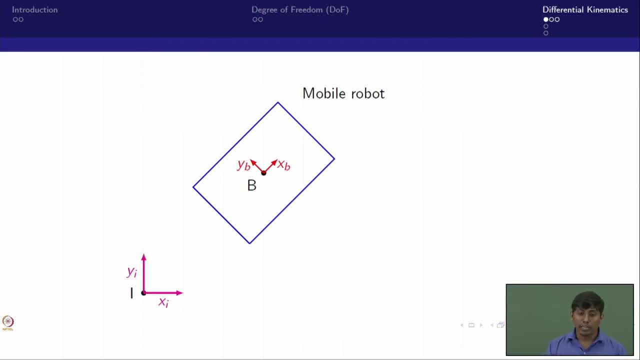 Since it is in a plane so I am not showing you. call z b and z i, So now you can see that I put one point b. another point is i, So definitely in a Cartesian way I can define the point b with respect to z. 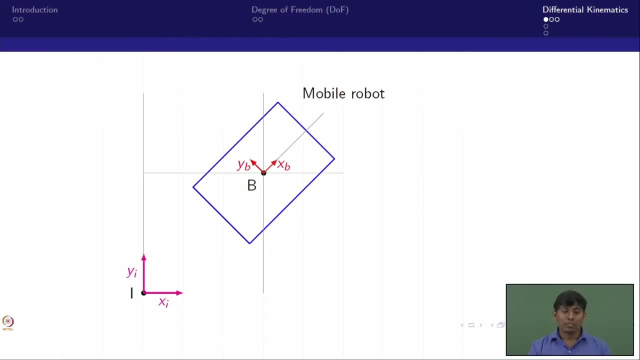 So what that would be. So I can actually like a draw imaginary line, I can actually like write it: x would be the x axis displacement or x axis position with respect to i, right So. and y would be the y axis position of b with respect to i. 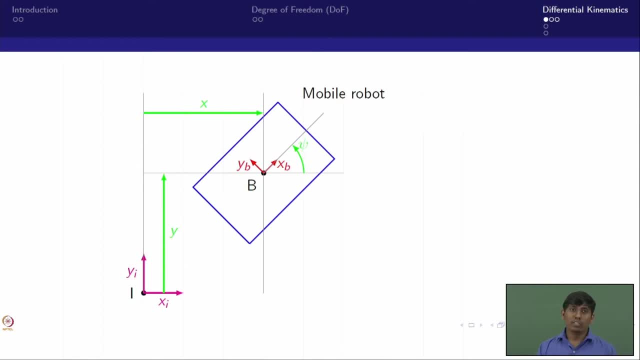 And I am putting another variable called psi, which is nothing but the rotation about z axis. Now you can see that I have already done right What I have done. I have actually like represent the point b with respect to the z axis. So that is b with respect to the fixed frame i. 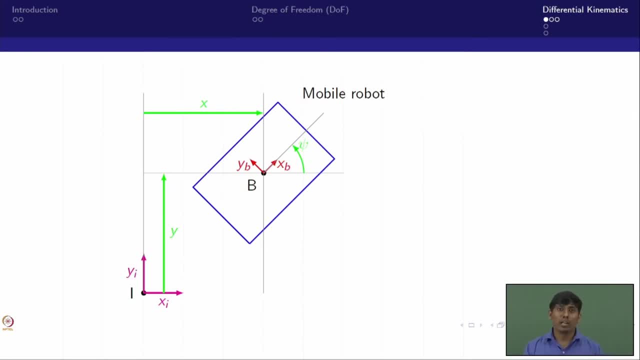 But what the issue comes, the mobile robot is actually like moving system And mostly what happened. the mobile robot would be connected with a wheel or leg that would be energizing the mobile base. For example, even you take a duster, the duster will not be having any input with respect to i. 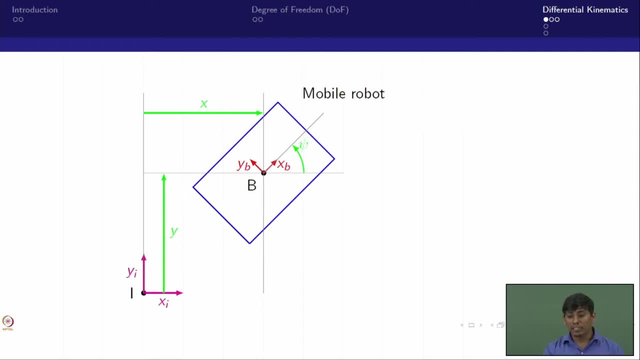 The input would be with respect to the b frame, In the sense what we know from the body frame. So there would be a longitudinal velocity, velocity which I am representing as u, and there would be a lateral velocity, which I am representing as a, v, and there is a angular velocity, which I am representing as r. So 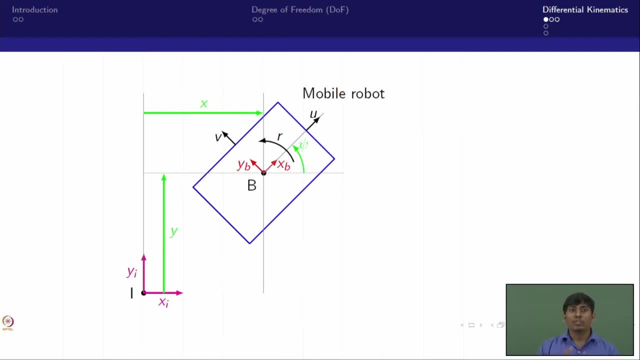 these are related with the body. ok, So now, if I take, b is instantaneously frozen. so now, what would be the instantaneous velocity of b along with xb, yb- that would be u and b- and what would be the instantaneous velocity of b with respect to zb, with this angular 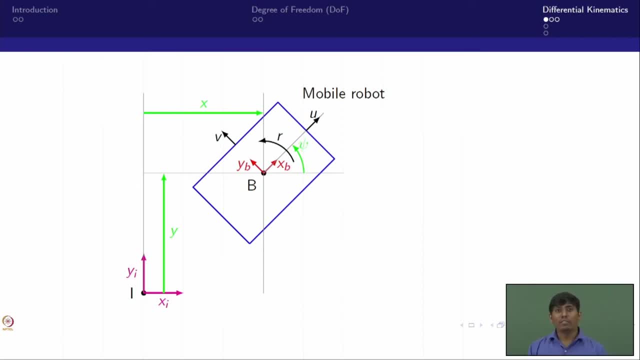 velocity, that is r. In the sense I have a instantaneous velocity, uvr, which I am assuming that this information is known with respect to frame b. but what I wanted, I wanted x, y psi, So how I will get. This is what the motion variable right, So how I will get. 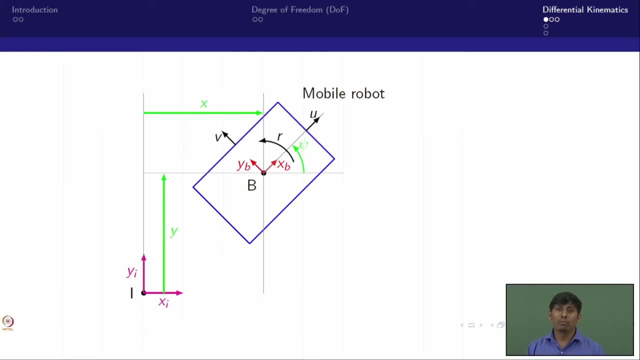 So you know the equation right: a equal to b. when this would be valid: a equal to b. when this equation is valid, both a and b dimensions are right and units are right. So in this case you can see that uvr is one set of variable. So x, y, psi is another set of variable. 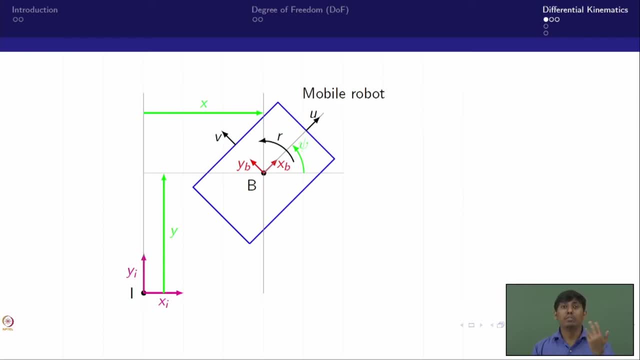 but you can see x, y, psi are, you can say, positional variable. there are linear position and angular position, whereas uvr is the velocity information in the sense linear and angular velocities, Both are actually distinct, So these are not straight away same. So then, 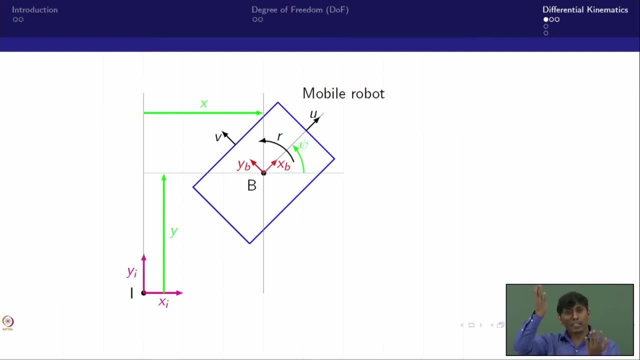 what one can see. Either you can actually like integrate that velocity, bring it to, you can say, positional domain, or you can actually like elevate the position by differentiating and bring it to the you can say time derivative In the sense what one can see, So you can. 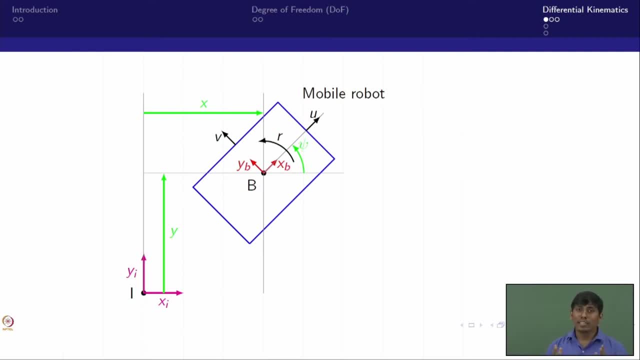 actually like do either one. So, which is easy, The instantaneous velocity is already instantaneous. I cannot get the instantaneous position Right, So obviously one can actually like see, So I can elevate the xy psi into x dot, y dot and psi dot. whatever I put x top of dot, that represent dx by dt. Ok, So this: 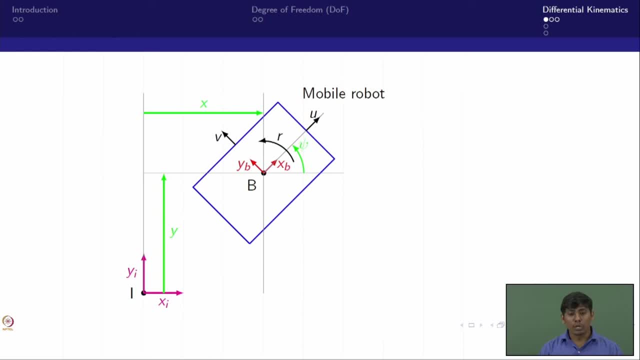 is what we are trying to see. So now you can see that the x dot, y dot and psi dot would be along with x axis, that would be x dot. along with y axis, that would be y dot. and about the z axis rotation, that is what psi dot. 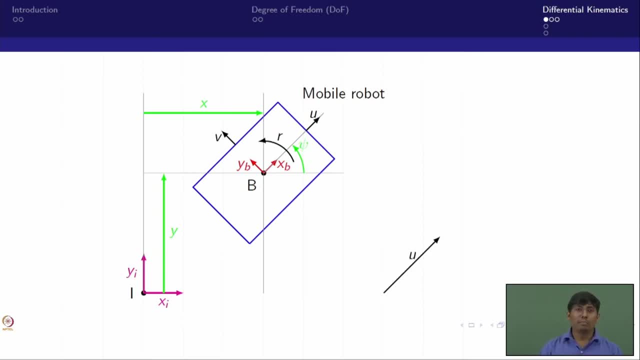 At what we have? u? vr. So now the? u can be actually like represented on the frame of I. So how we can represent it, So we can project so la of cosine. So now I am actually like taking the? u and projecting on the frame. you can say I. So now what would? 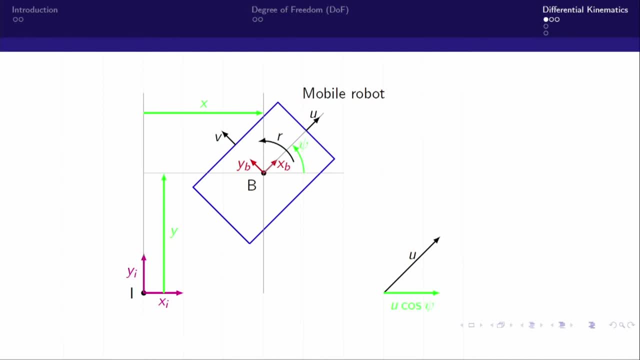 be there The angle already. I know psi. So if I projected on the x axis that would be equivalent to u cos psi. If I projected on the y axis that would be equivalent to u sin psi. Ok, So now, similarly, I take V vector. So if I actually like, projected on x axis and y. 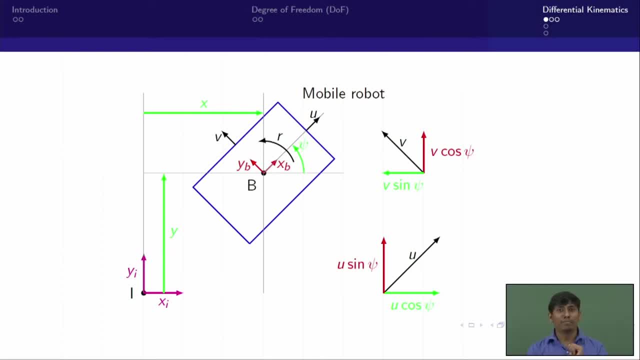 axis, it is V sin psi and V cos psi. So now I projected. So then, why you projected? So this is one of the question will come Now. since the system is, you can say static at instantaneous point, in the sense, whatever the motion happening on the B, if I actually 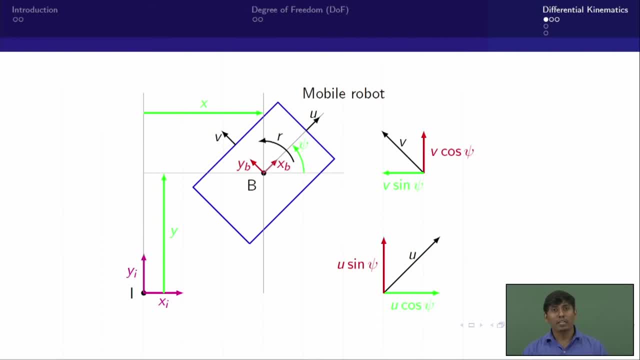 like C with respect to I. that supposed to be same right. So in the sense you can see that whatever the longitudinal velocity, which is u cos psi and V sin psi, the vector addition supposed to be equivalent to x dot. that is what we are doing it. So I am taking u cos. 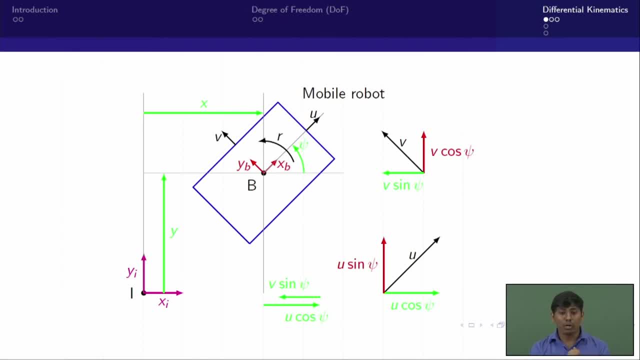 psi and V sin psi. I am doing the vector addition. what would be? that is what x dot. Now, similarly, you can see y axis vector addition vectors. So u sin psi and V cos psi. that is what I am doing. So if I take vector addition, that would be equivalent to y dot. And what? 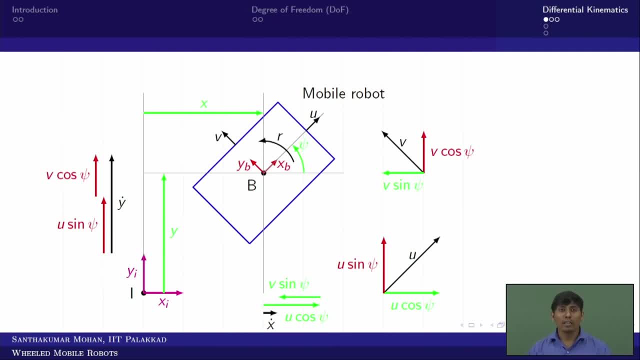 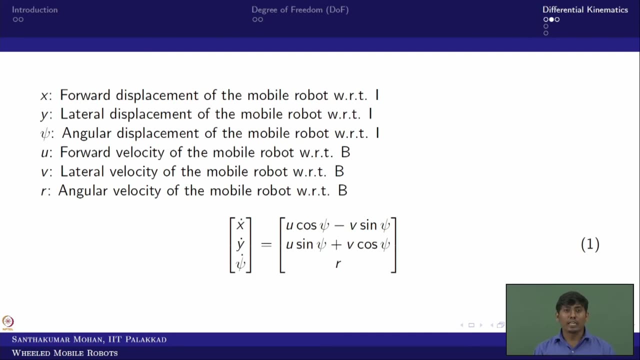 one can see easily the psi dot and r are actually like in the same. you can say direction and as well as it is parallel. So in the sense r is straight away equivalent to psi dot. So in the sense, what one can see? So x dot, I can write as u cos psi minus V, sin psi and. 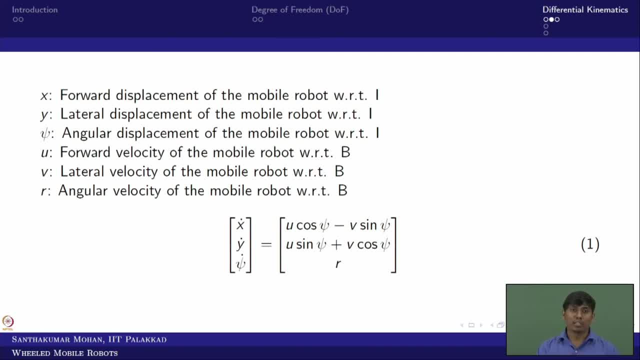 y dot. I can write as u: sin, psi plus V, cos, psi and psi dot. I can write as r that I am writing in a vector form. You can see this particular slide. So x, dot, y, dot, psi dot. I am writing as a one of the vector that later on I am going to. 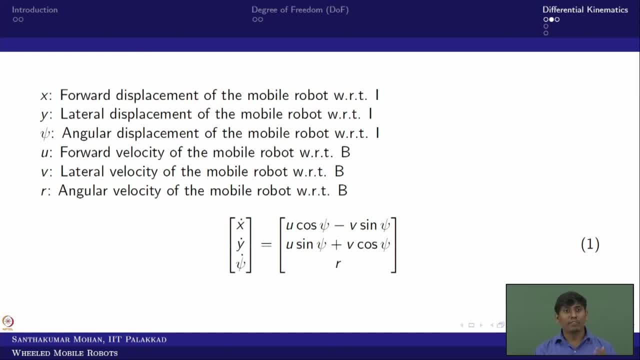 call as eta dot, So where eta is vector of x, y and psi. So eta dot is actually like x dot, y dot and psi dot. that is equivalent to u cos psi minus V sin psi, u sin psi plus V cos psi and r. So now what one can see. I can actually like group it this u V r into: 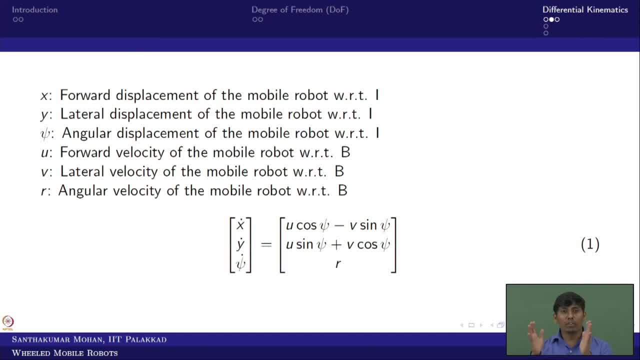 y dot and x dot, y dot and psi dot is another side. So whatever the in between, that is what you call mapping. So now what you can see, u V r is the body fixed instantaneous velocity and x dot, y dot and psi dot is the initial fixed time derivatives of the generalized 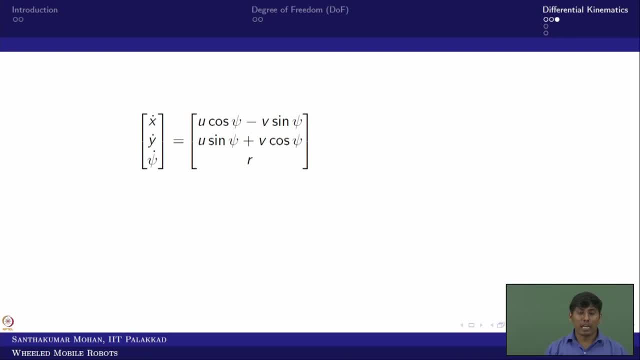 coordinate. Now I can map. So this is what the next slide is telling. You can see, this is the relation. I got it and I am rewriting into a matrix and vector form. So what one can see? I can map x, dot, y, dot, psi dot with respect to u left. So here you can see I 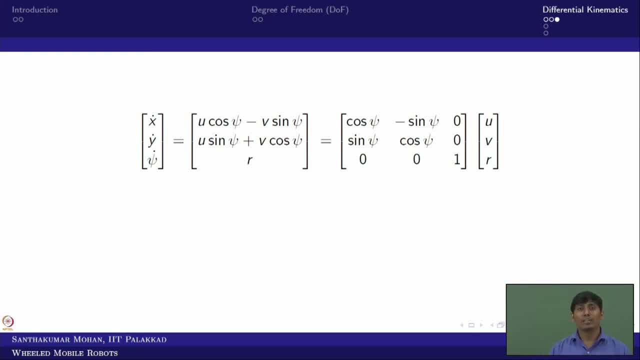 respect to uvr. So this is what we call kinematic relation. So this is what the kinematic model. So now this particular matrix I am going to call as one of the generalized matrix called mapping matrix, Some people call kinematic transformation matrix. but this kinematic 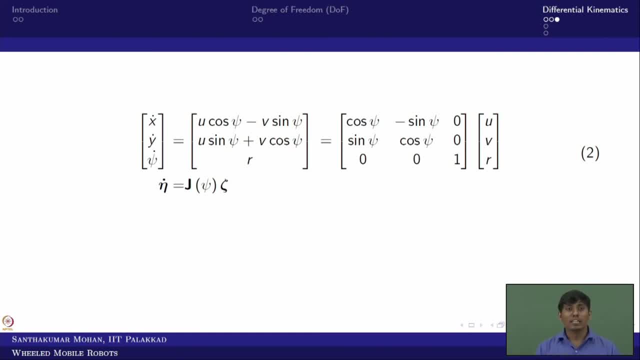 transformation has actually like, given in time domain, in the sense time derivative domain, given by Jacobi, So this particular matrix called Jacobian matrix, So now J of psi, what you call Jacobian matrix, What this particular relationship is giving a idea where you consider 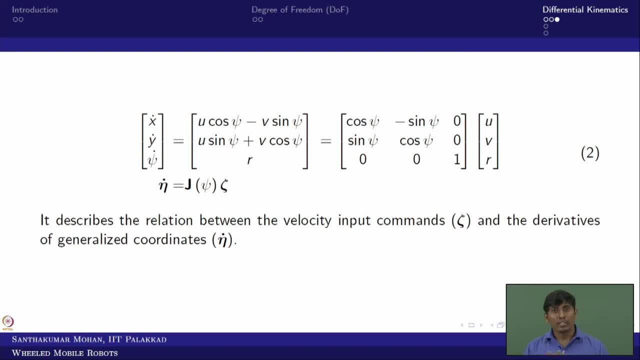 uvr as one of the vector called zeta. that is what? nothing but velocity input. So now you assume that this is the command. So now velocity input command is mapped to the you call the time derivatives of the generalized coordinate eta dot. So now you can see that. 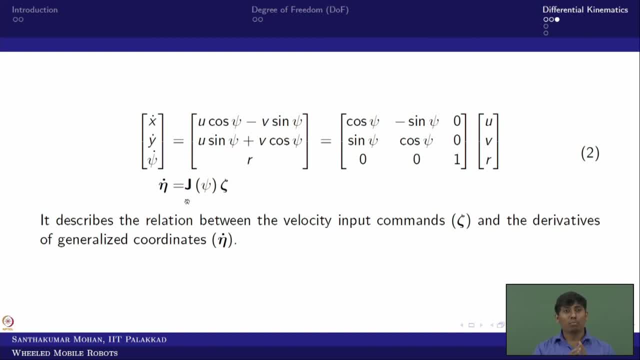 this is mapping between these two, right? So that is what we call mobile robot kinematic equation. Now, what you obtain? this equation, nothing but the robot kinematic equation. So, as I already told, robot kinematics means not only study of motion, it is mapping further. 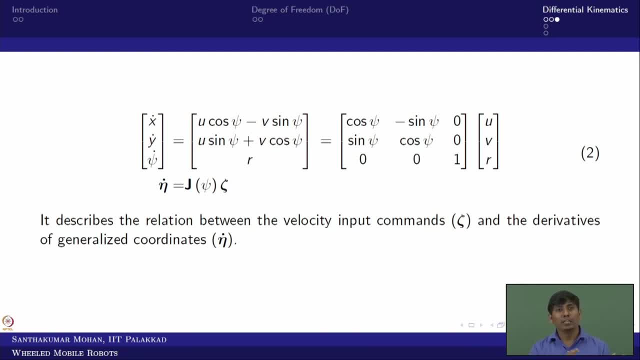 right. So now you can see that the mapping between happening either actually like velocity input command to the time derivative of generalized coordinate. So now, based on that, it can be classified into two. ok, So what that mean? So one is actually like you give input command. 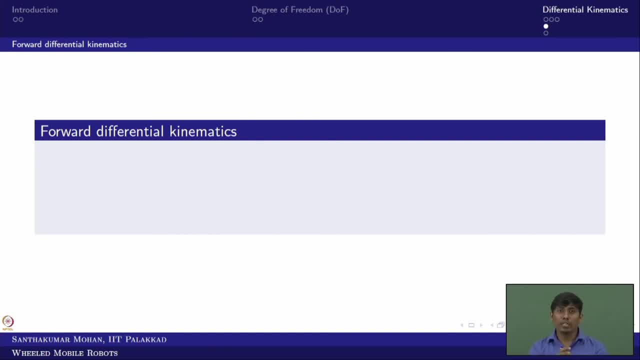 velocities or input velocity command. you give it In the sense you take the mobile robot, connect the wheel and connect the motor and run the motor with certain speed. So what you will see, You will see how the robot moves right. So, in the sense, what you are trying to understand, you are giving the input command and seeing. 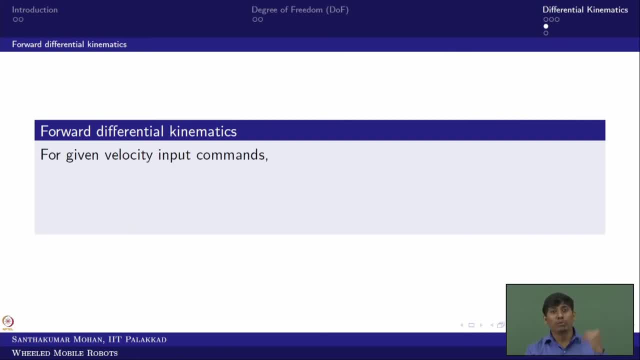 the, you can say the time derivative. and if you integrate that, what you will get? the generalized derivative, you can say generalized coordinate. So this is what we are trying to see for a given velocity input command: finding the derivatives of generalized coordinate, nothing but finding the system motion. this is what you call forward differential kinematics. 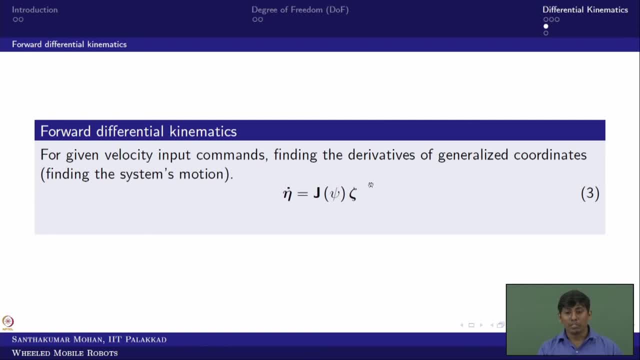 So why it is so called forward? Because your input is straight forward given and you are seeing the motion variable how it moves. So this is nothing but one scenario. if you are doing mathematically, it is try to simulate. you take a real robot and do it, nothing but. 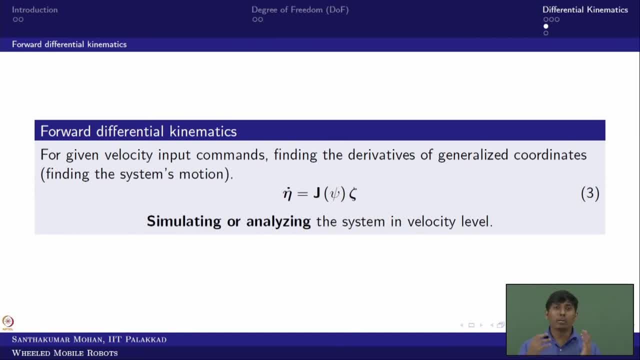 analyzing, right, So that is what we call. So simulating or analyzing the system in velocity level, that is what forward differential kinematics. So now, what would be the next case? So you just imagine. you just imagine. So you are having some desired derivative of 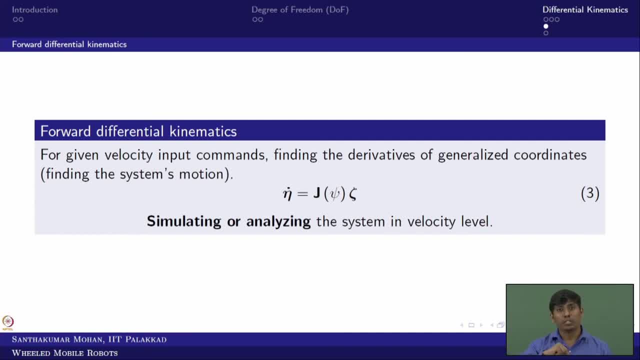 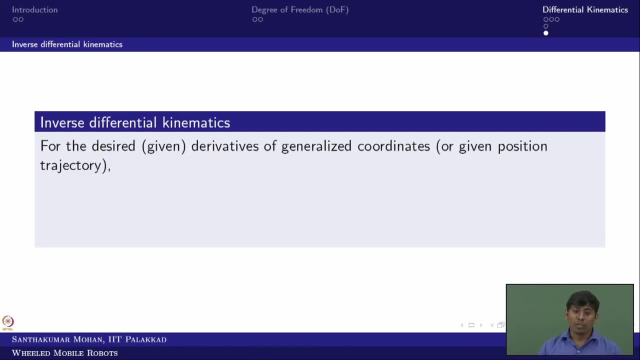 generalized coordinate, you want to see what would be the input. So in the sense you are trying to do the reverse way. So that is why it is called inverse differential kinematics, where you can see that for a given you can say desired derivative of generalized coordinate. 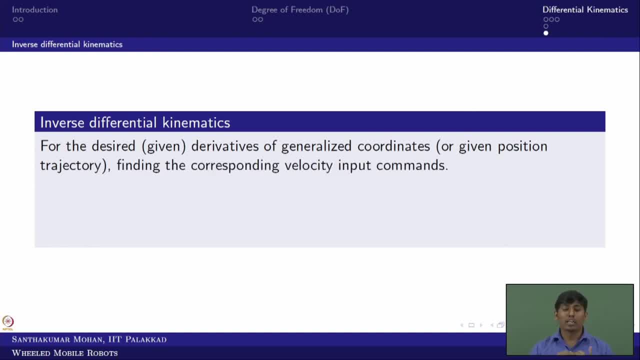 you are trying to find out, you can see that corresponding velocity input command. In the sense, what you are trying to see for a given position trajectory, you are trying to see what would be the, you can say, body fixed velocities. So this is what we call. 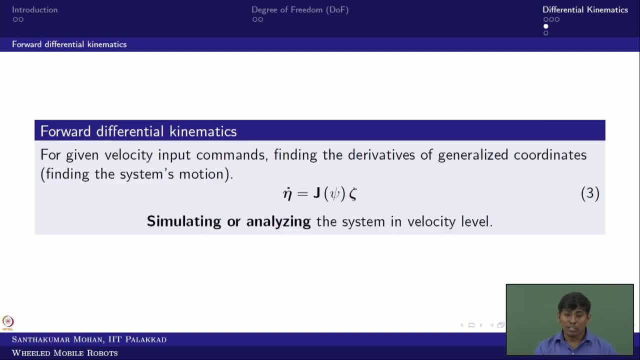 you can say inverse differential kinematics. you know already the equation. you see, eta dot is straight away Jacobian of. you can say J of psi into zeta. Now we are trying to find out the zeta. So obviously, what one usually? you see, this is known and this is. 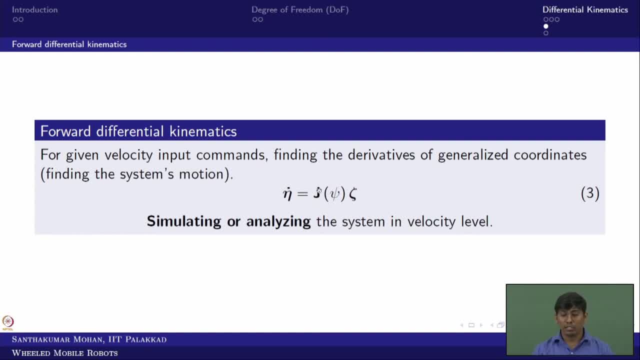 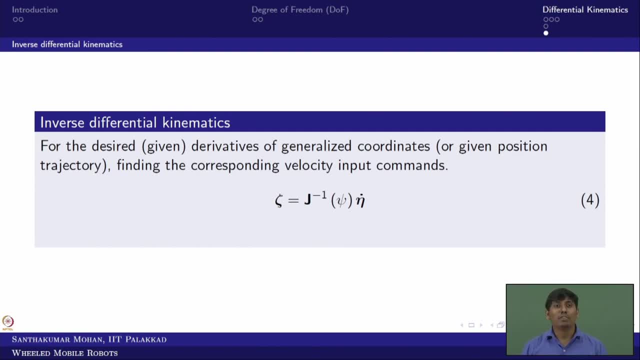 actually like: known and this is what unknown. So you take the inverse of this, So that is what we are doing it. So you can even imagine that this is known and this is unknown. So you can even imagine that this is a way you can actually take a remember that inverse. 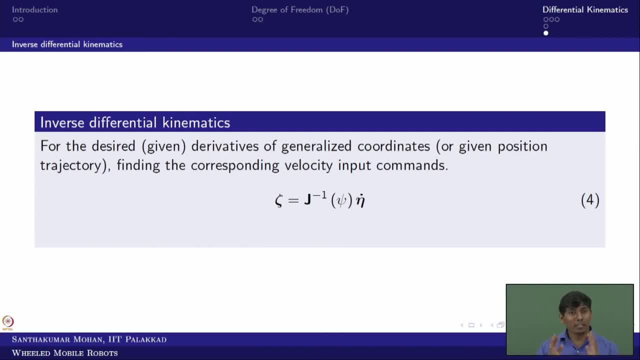 means J inverse will exist. Right? This is a blind. this is not right, but I can actually give an idea. So zeta is J inverse of psi into eta dot. So now what we are trying to see: The given I already mentioned, given decide So in the 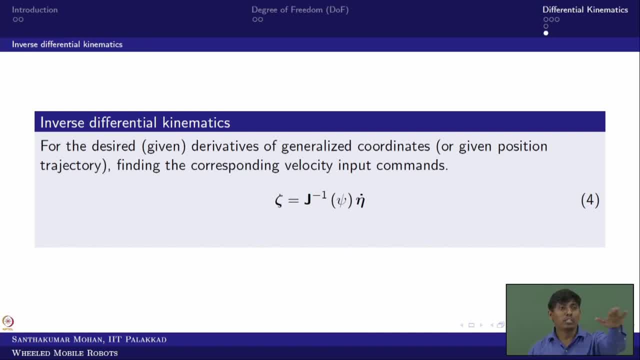 sense what we are trying to see. I want the robot, suppose suppose, to move in this manner. I want certain motion. this way Can I actually like make it In the sense what we are trying to see. So the robot suppose to move. So I think that I want the robot to move straight. shave prove. 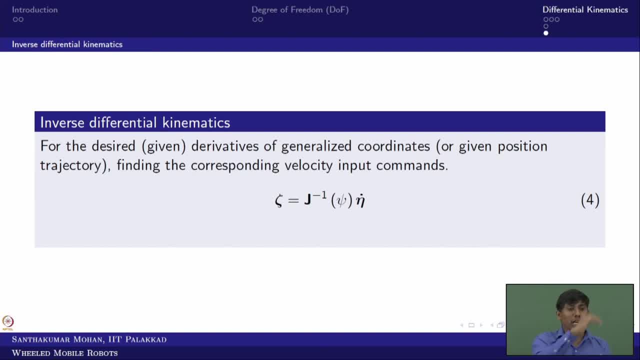 that robot if it moves straight in to this point And in this way I want certain motion. this way Can I actually make it. in the sense, I am attempting to act upon the drawing, do it quickly. I am trying to navigate in particular way, So in the sense, what you are trying to do. 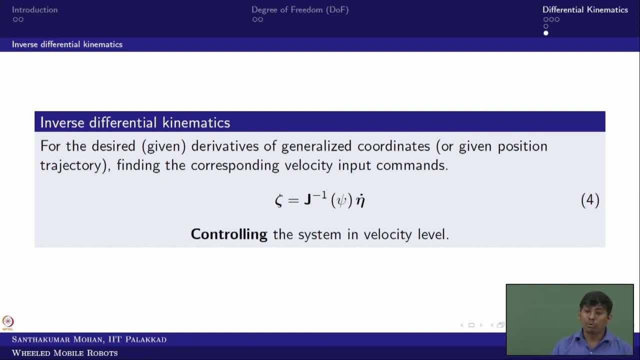 You are trying to do a controlling action, right? So that is what you call controlling the system in velocity level. So this is what the inverse differential kinematics Further on this inverse differential kinematics, what we call control, The control can be open. 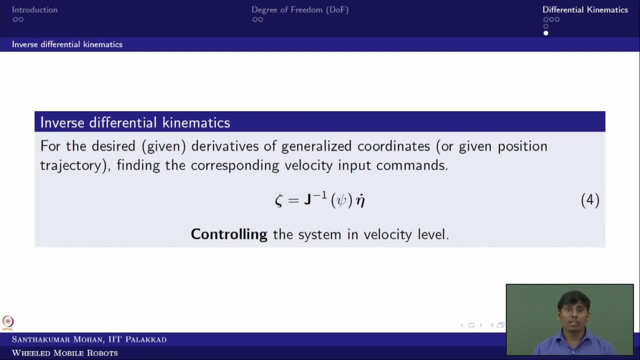 loop In the sense you just take eta, dot and j inverse of psi. This is actually like very open, but you can actually like even make a closed loop. You take a feedback and make it. Then that is actually like feedback control. But these all we would be seeing in the end of this course. 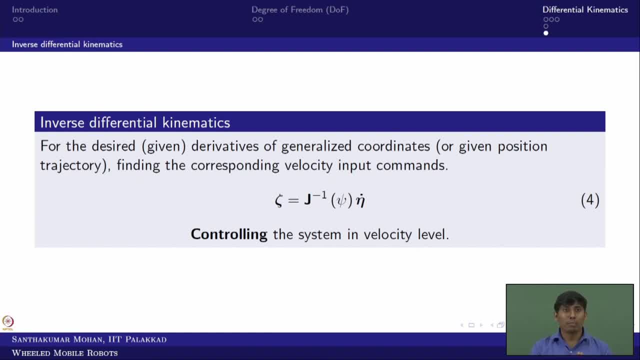 But right now what you understood is actually like what is mobile robot kinematics? It is nothing but mapping between two. you can say velocity spaces, So one is actually like input. you can say velocity input commands, So the other one is derivative. that to time derivative. 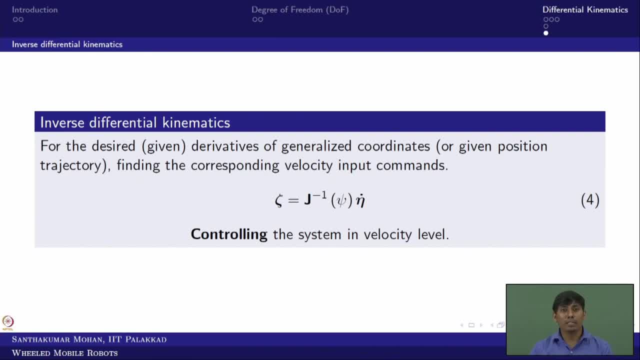 of generalized coordinate. You are trying to map Why it is mapping, Because in mobile robot it cannot be directly find it. So you have done with the mapping. So this is what the mapping further divide into two. So one is forward differential kinematics. 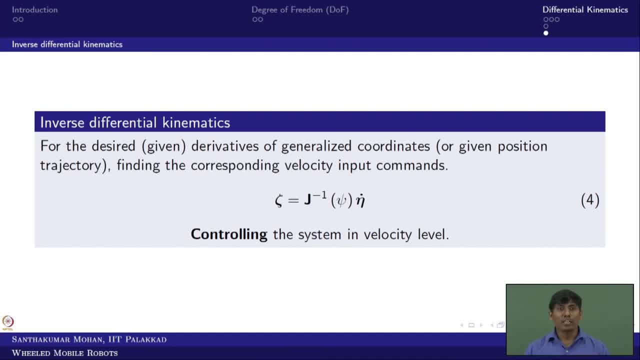 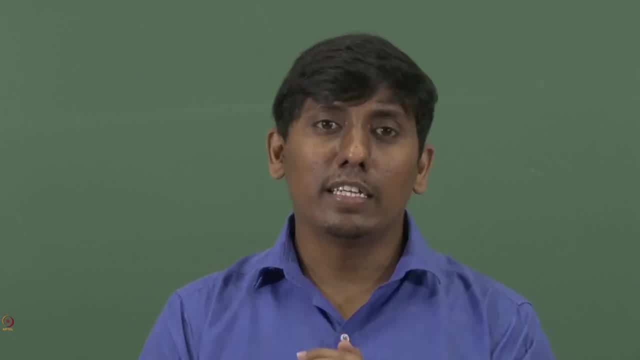 another one is inverse differential kinematics. In the next lecture we will see how the zeta is obtained, Because the zeta is actually like a slightly different right, Because the zeta is actually like what you call velocity input commands. The velocity input commands is actually 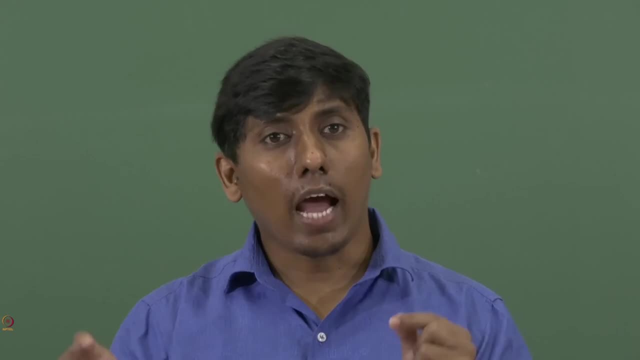 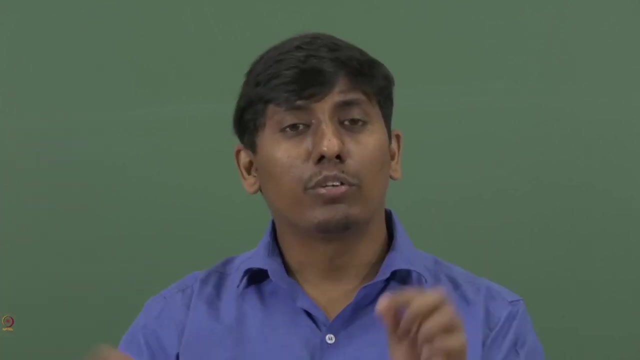 like coming from the wheeled configuration. So then we have to bring one more mapping where the zeta would be coming with. you can say angular velocity of the wheel. So that is what we are trying to address in the next lecture. So before that, probably we will see the one of the important aspect you should. 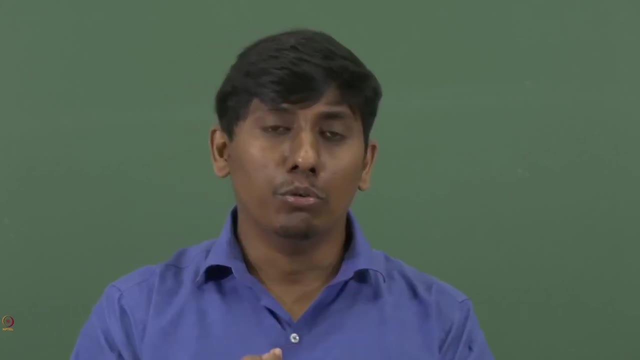 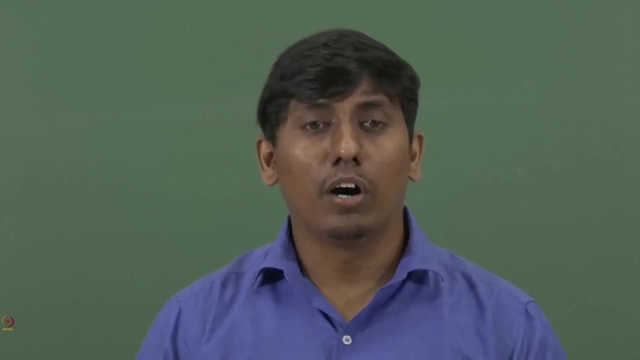 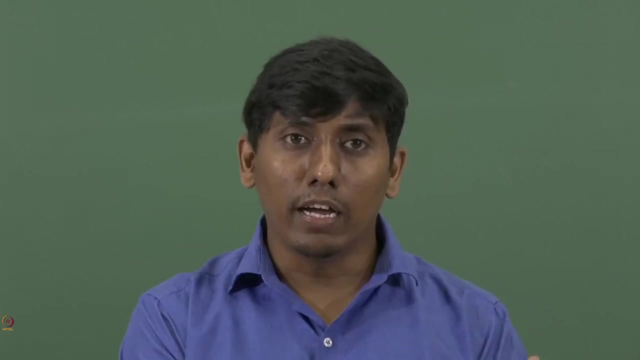 know, like what are the types of wheels which are used in the mobile robot, how that can be classified and how we can actually like make it. In the sense, the next slide or next lecture would be talking about more about a real mobile robot. So right now we talk about degree of freedom, but since it is a mobile robot, the maneuverability 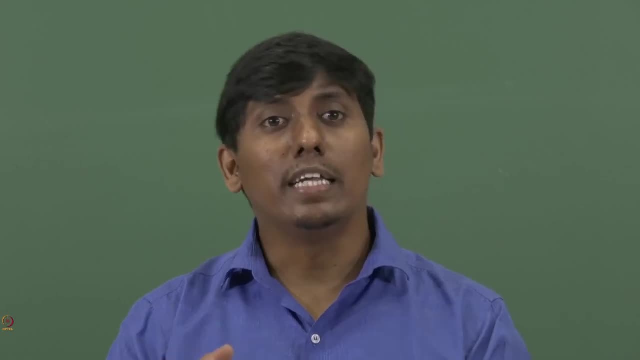 will come into a picture. So the next lecture would be talking about degree of maneuverability and we will see how to obtain that. So, based on that, the further lecture will come about: the wheeled. you can say locomotion, in the sense you will be bringing the kinematic relationship. 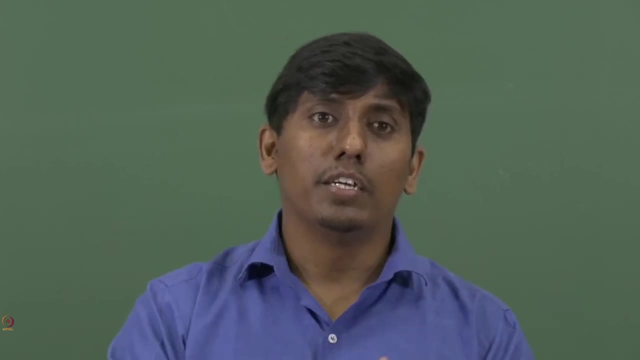 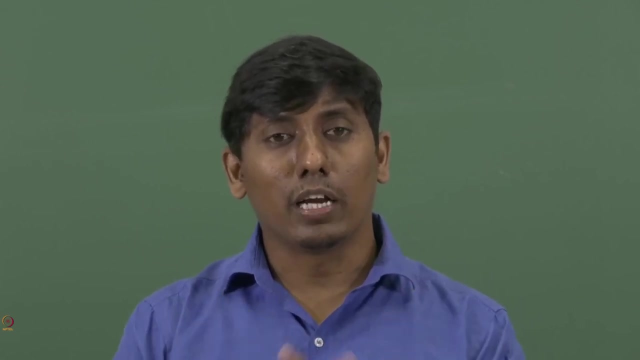 between the angular velocity of the wheel to the input command velocities, and then you can make it to the time derivative of generalized coordinate. So with that you can see that this particular lecture 3 is over. So then lecture 4 would be talking about types of wheel, and then lecture 5 would be talking about the kinematic simulation. 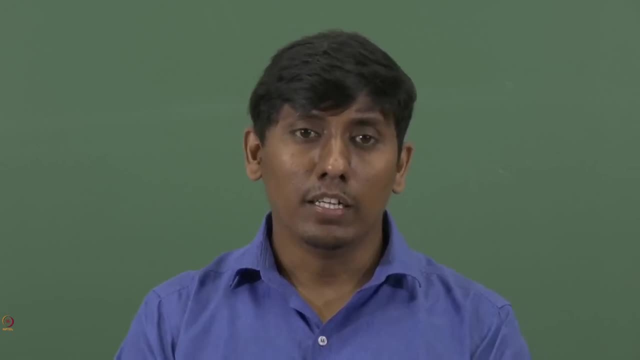 So with that we would be finishing this course here. So we will see in the lecture 4 later. Bye, Thank you.